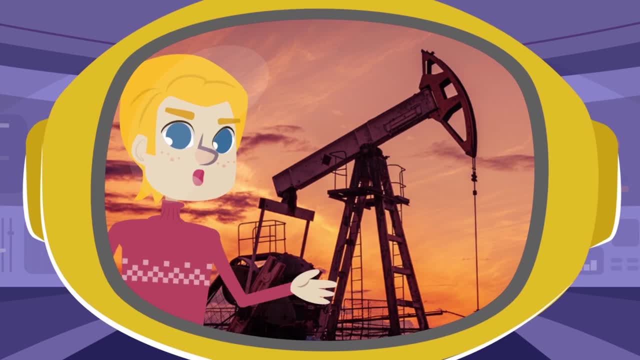 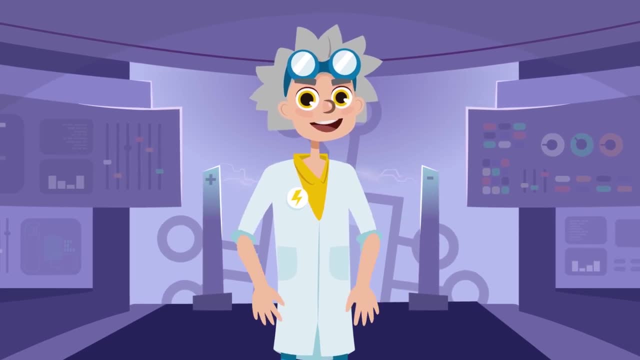 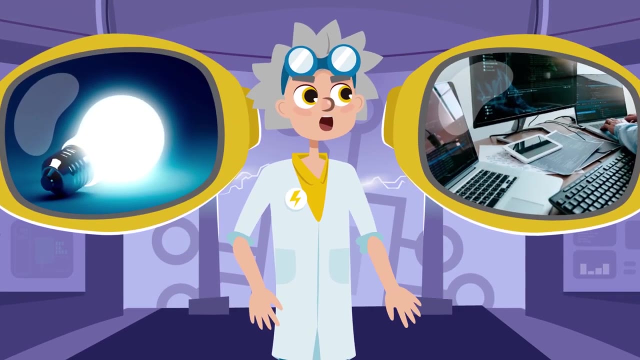 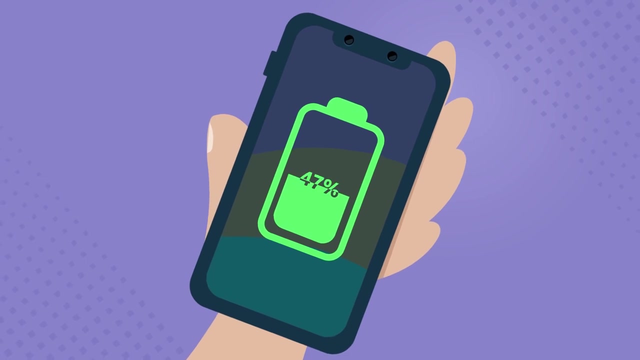 and electricity, Oil or even the sun. Thanks, guys. I think we learned a lot from our friends. As we saw, electricity is a type of energy we use to turn on lights or power our electronic devices. Electricity has become so important in our lives that we can't imagine living without it. 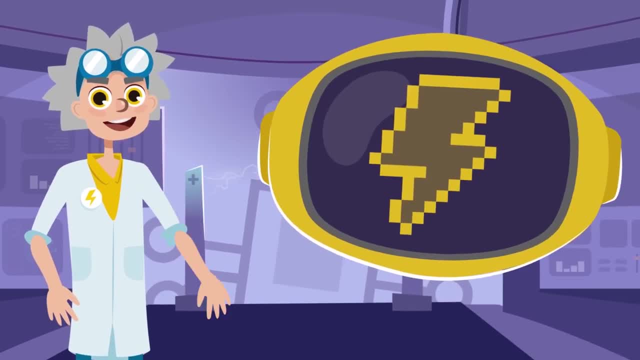 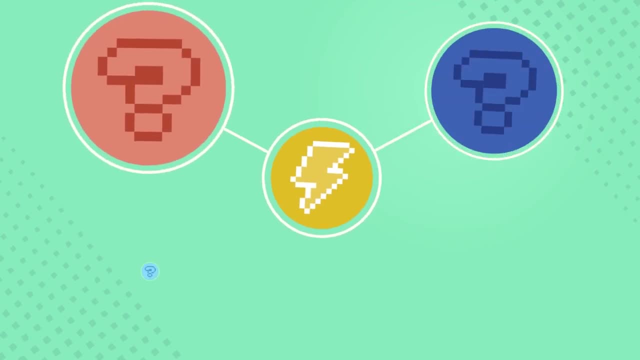 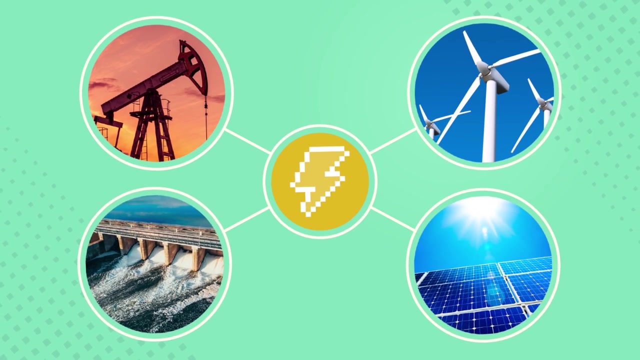 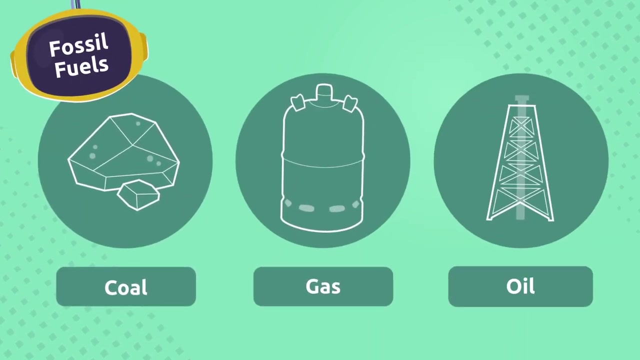 As our last friend said, electricity can be produced in many different ways. Let's find out. We can use energy from natural resources like fossil fuels, wind, water and the sun to create electricity. Let's take a look. Fossil fuels such as coal, gas and oil are natural resources found beneath the Earth's surface. 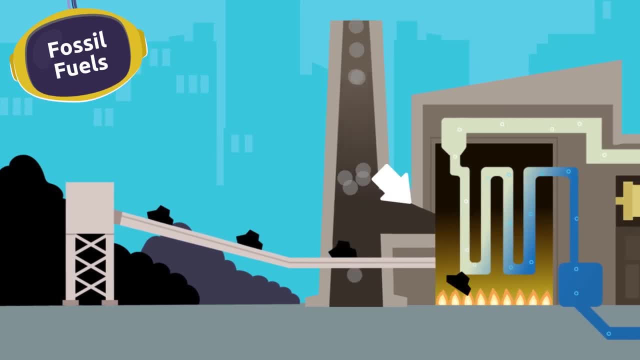 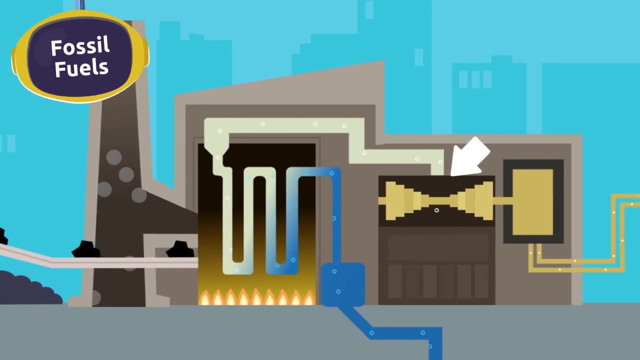 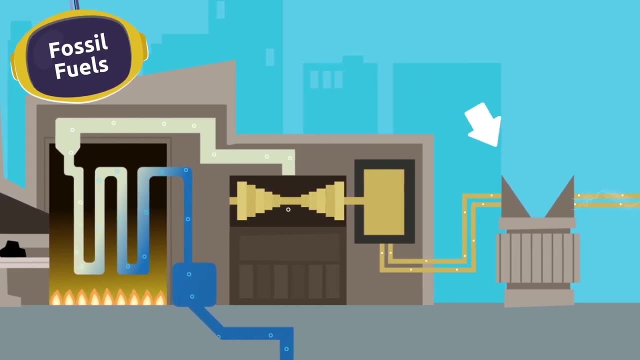 We burn these fossil fuels at power plants to boil large amounts of electricity. This produces steam that is powerful enough to turn a large turbine, which basically looks like a big egg beater. When the turbines turn, they activate a generator that produces electricity. 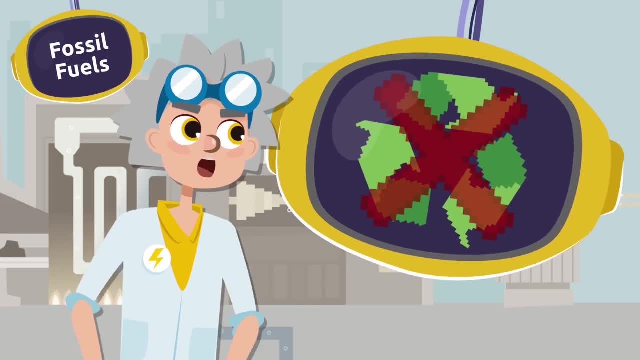 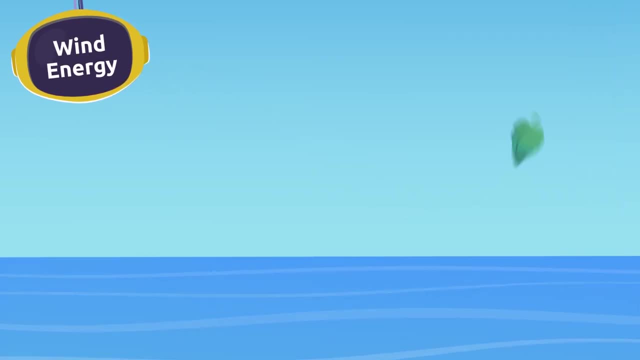 But we have to be careful, because producing electricity with fossil fuels is harmful to the environment. Another way we can get electricity is by using the forces of nature. This is by using the force of the wind, In other words, wind energy. Have you ever seen wind turbines? 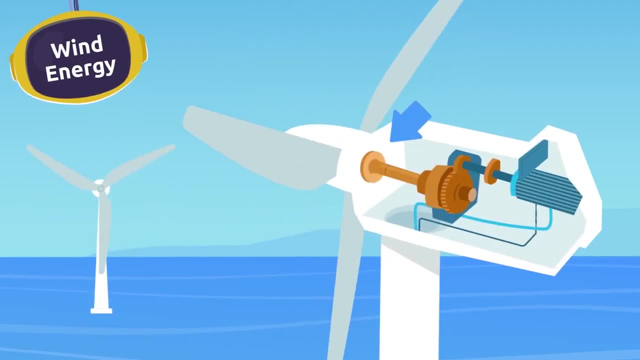 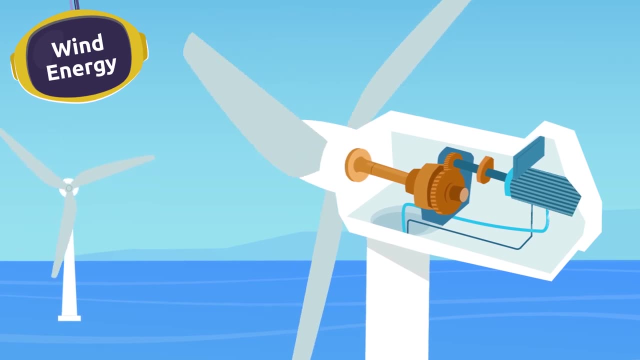 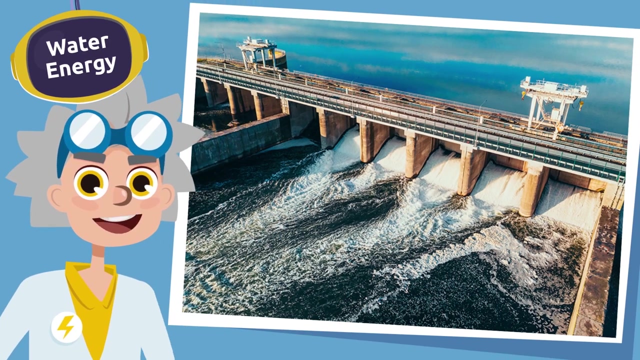 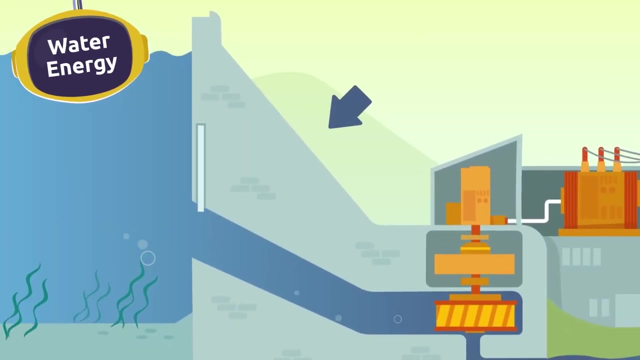 When the wind blows and pushes the blades of the wind turbines in a circular motion, it also turns a shaft, which activates the generator producing electricity. We can also get energy from the force of the water. Maybe you have seen a dam. It is a big wall built to collect large amounts of water. 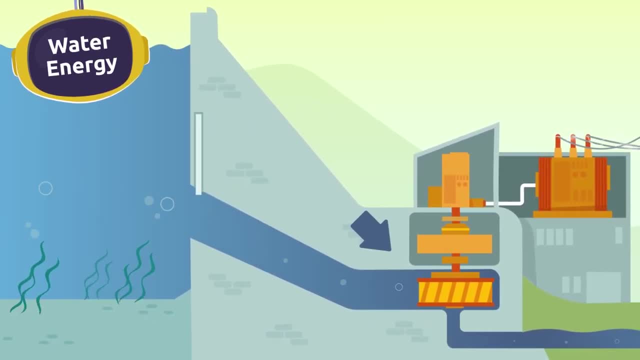 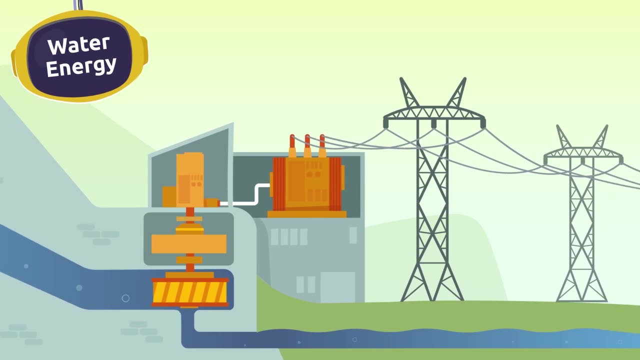 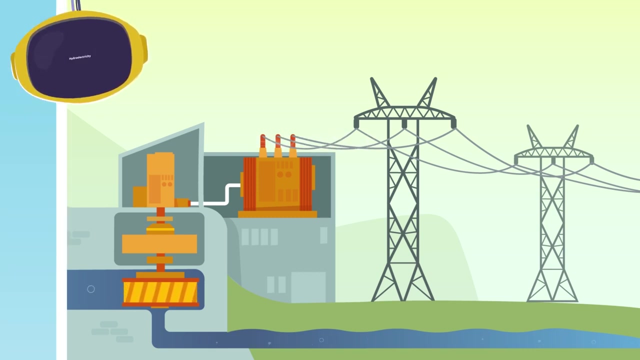 The water is pushed through pipes, which creates the pressure needed to turn the blades of the turbine, thus activating the generator and producing electricity. This type of energy is called hydroelectricity. Lastly, we will talk about the energy we can use from the sun. 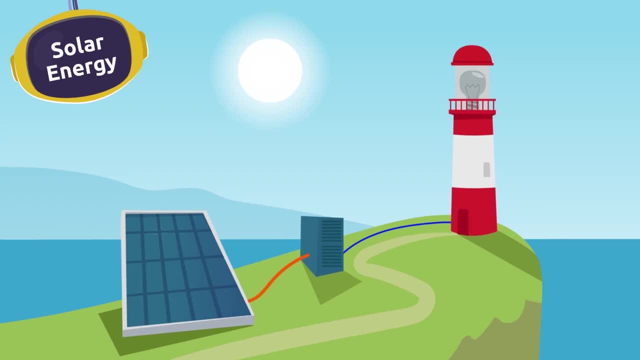 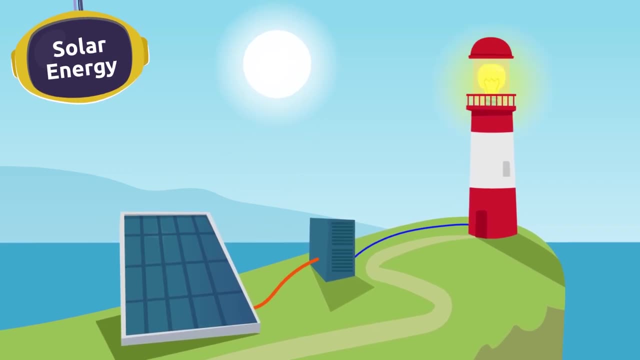 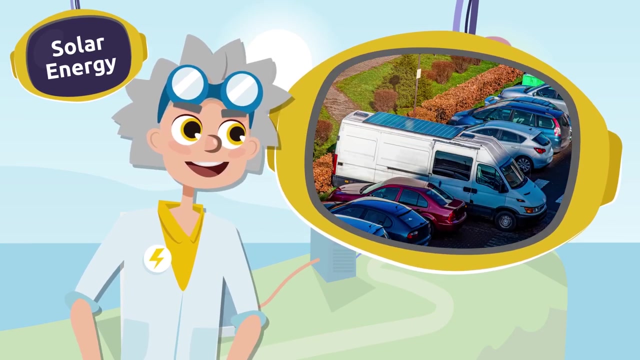 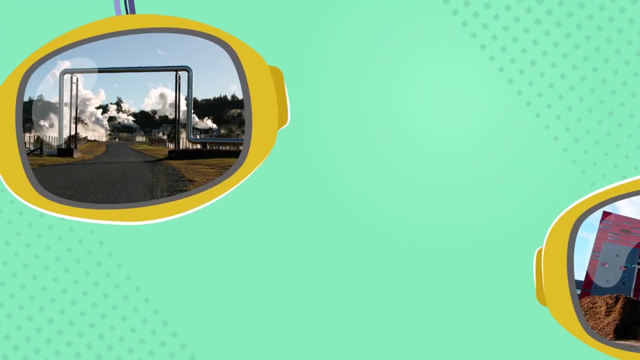 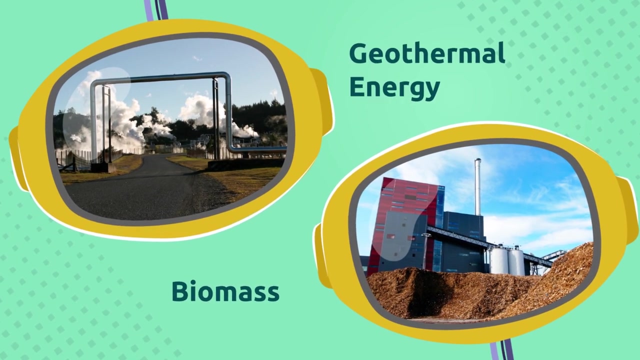 This is called solar energy. When it is a sunny day, the solar panels capture the solar energy from the sun and transform it into electricity. Solar panels can be found on buildings, cars, boats and space satellites. There are more ways to produce electricity from these natural resources, but the ones we saw today are the most common. 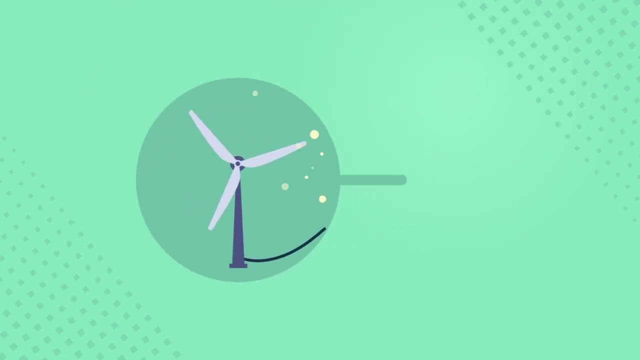 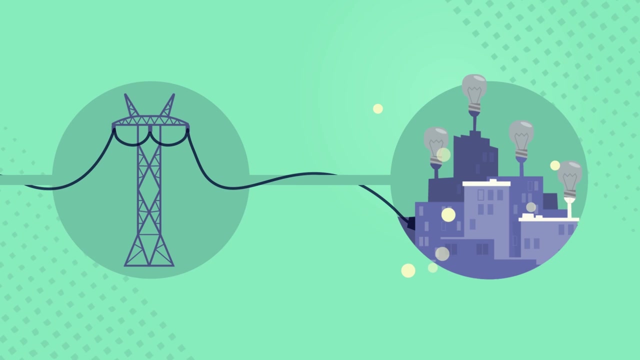 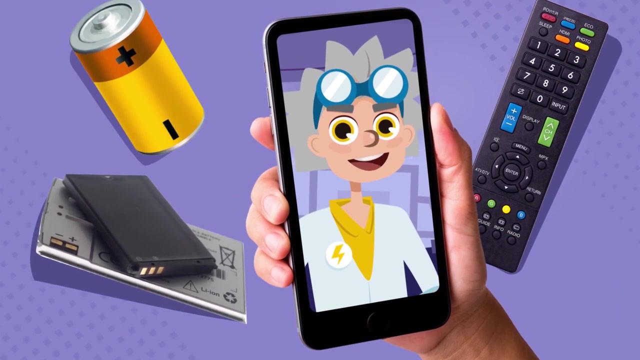 Once the electricity is created using these natural resources, it is then transported through cables and wires to our homes, schools and workplaces, ready for us to use. Electricity can also be stored in batteries that we use to power our flashlights, mobile phones or remote controls. 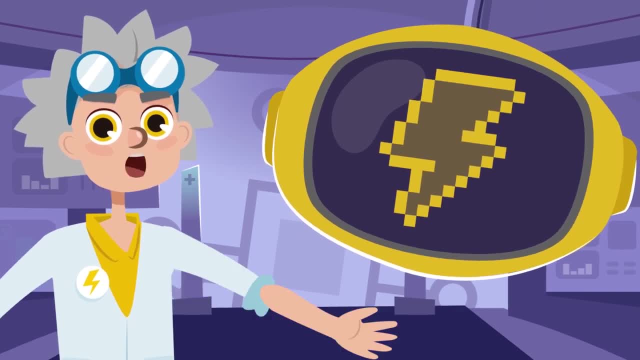 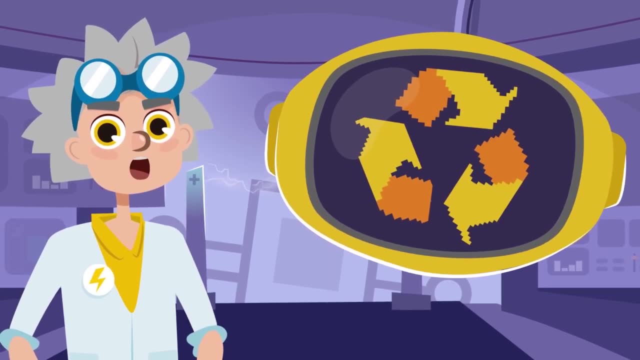 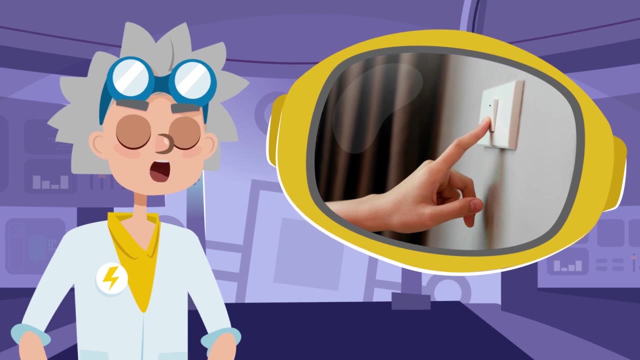 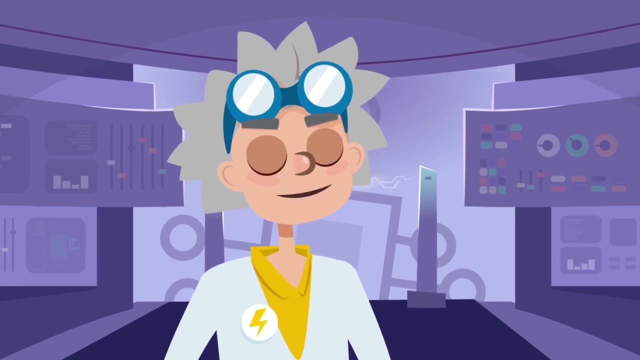 Well, there you have it. Now we know where our electricity comes from. It's important to understand that electricity should not be wasted. Remember to turn off the lights and other electrical devices when they're not in use. Up next, we're going to discover types of electricity and circuits. 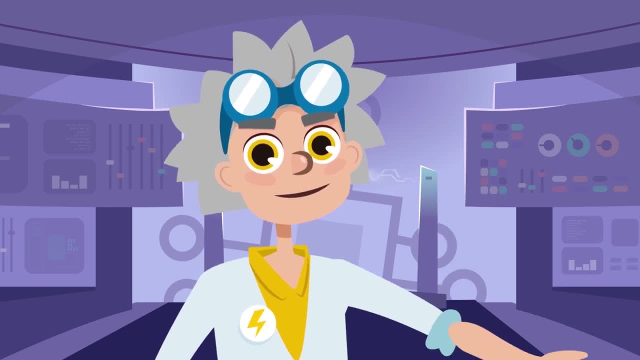 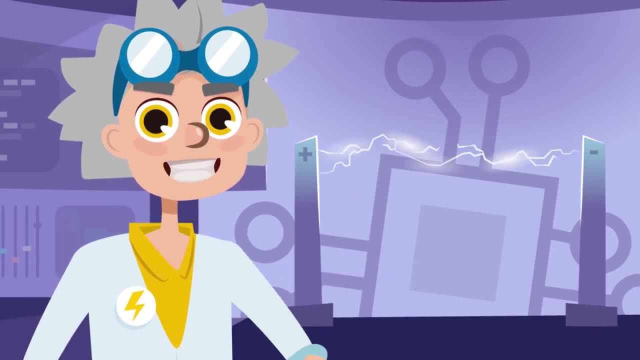 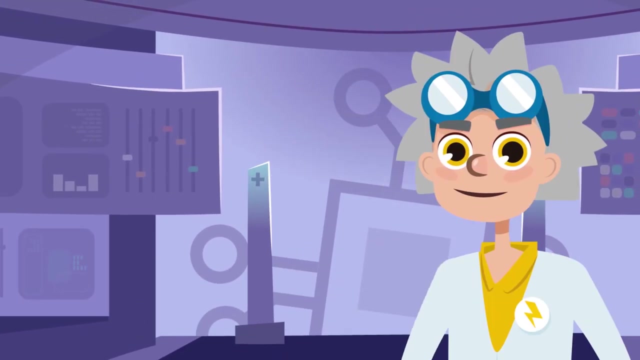 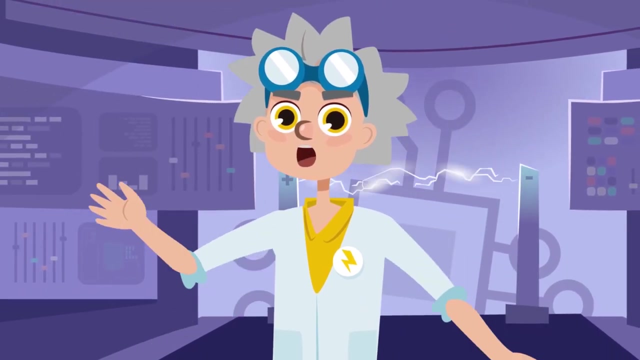 Stay tuned for our next video. Hey friends, Welcome back to Science Madness, A program where we discover, learn and experiment new things. In our last video, we learned what electricity was and where it came from. Today, we're going to learn about types of electricity and circuits. 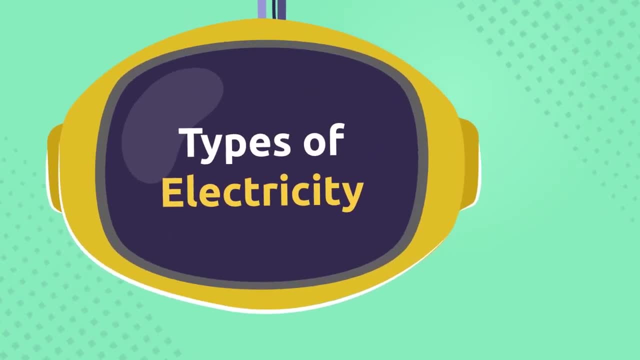 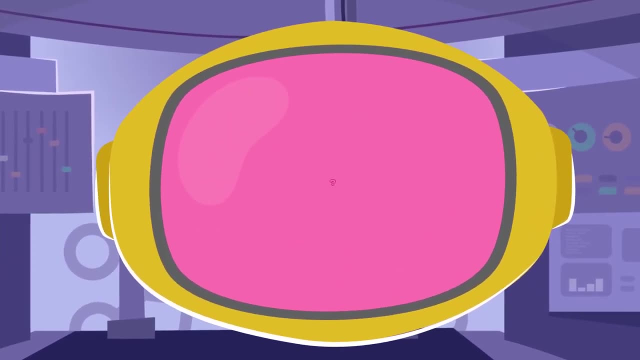 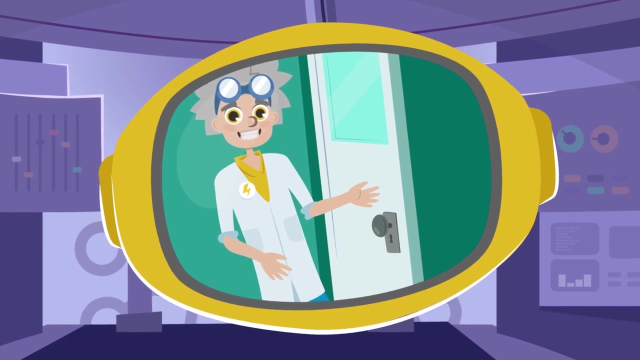 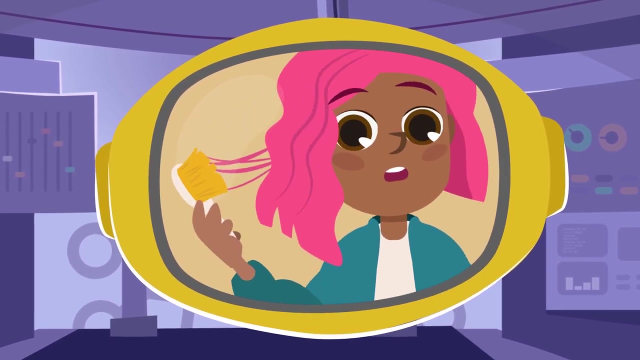 Are you ready? Let's start with a couple of questions. Have you ever walked across a carpet And later felt a small shock when you touched an object? Yes, And have you ever brushed your hair for a while and noticed how it got stuck to your brush? 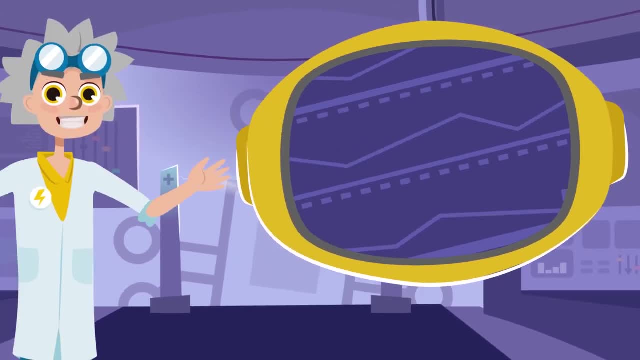 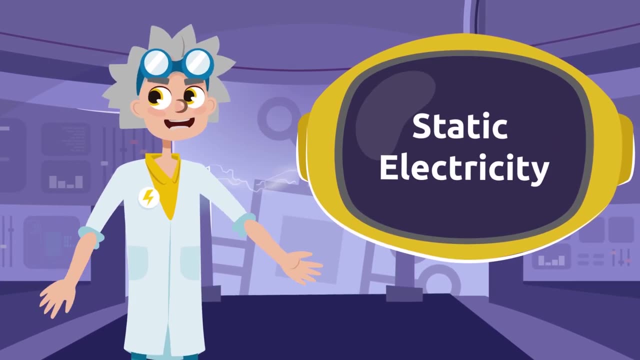 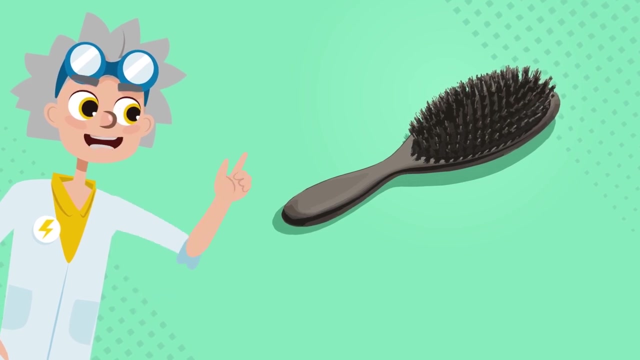 Yes, Good. Well, this happens because of static electricity, meaning that an electric charge is created when objects rub against each other. So let me explain. All objects are made up of atoms that are impossible to see because they are super small. 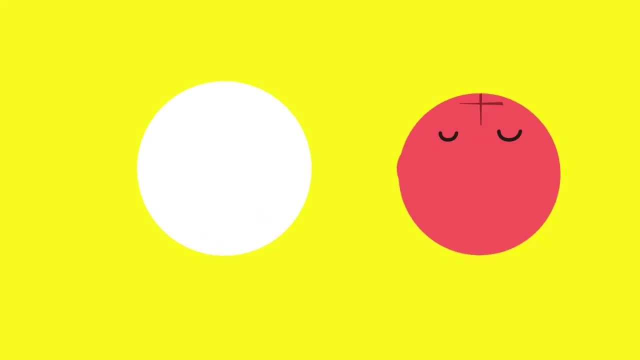 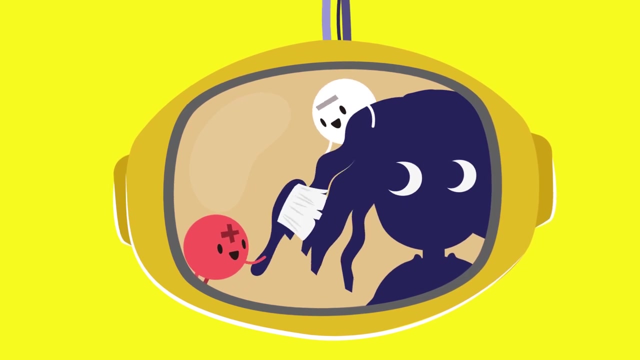 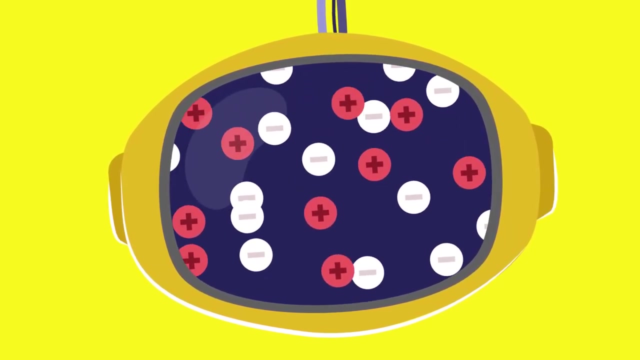 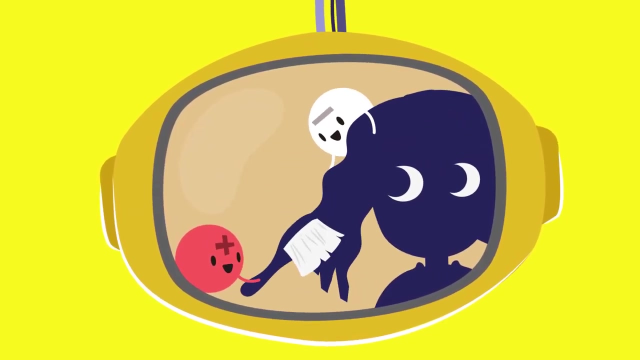 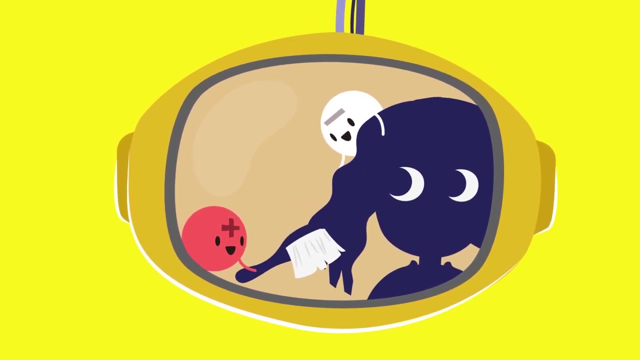 These atoms have different electric charges, positive or negative. When two objects rub against each other, they become charged with energy and the positive and negative charges move, creating an imbalance. We call this imbalance static electricity. Sometimes static electricity causes two objects to stick together or attract to each other, such as hair and a brush when we comb our hair. 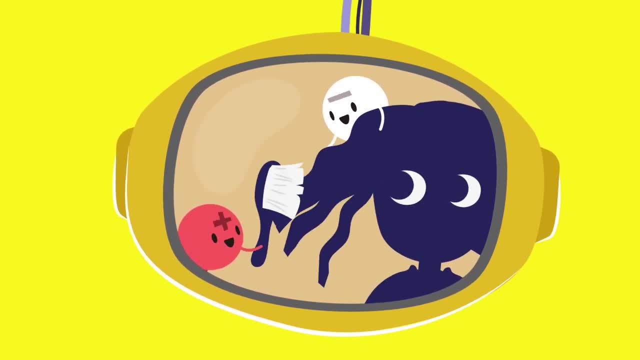 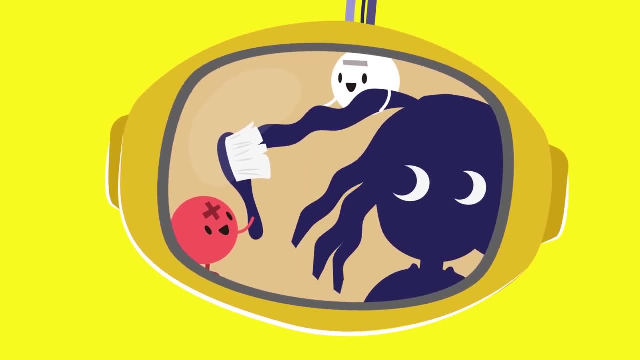 The brush has more positive charges and the hair has more negative charges. Positive and negative charges really like each other. That means they attract each other, Whereas atoms with the same charge don't like each other at all, Which is why you will notice that they don't like each other. 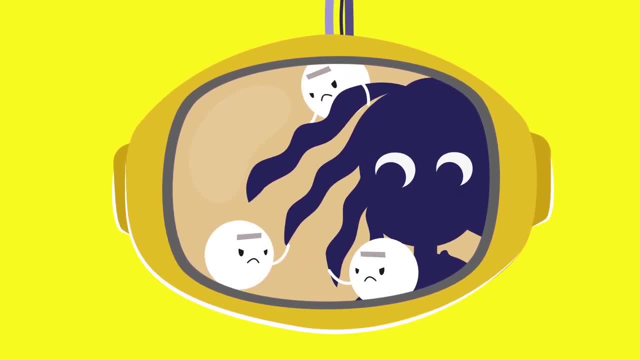 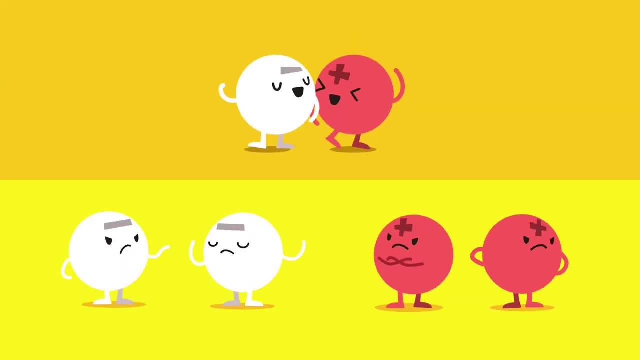 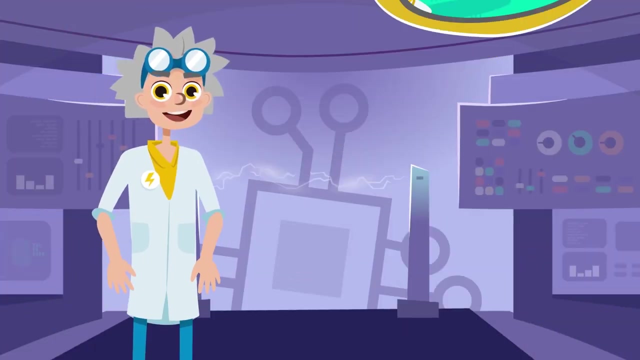 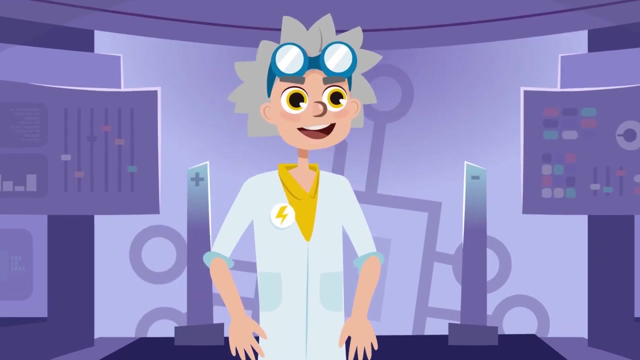 This is because each strand of hair is negatively charged. When two objects have the same charge, either positive or negative, they either move away from each other or repel each other. Now we know why sometimes some objects give us a shock. It's because we send the excess electrical charge from one object to another. 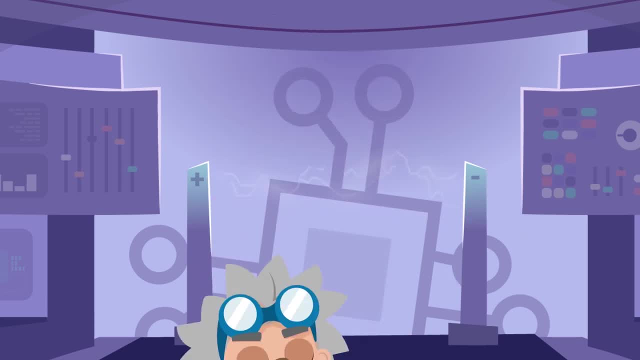 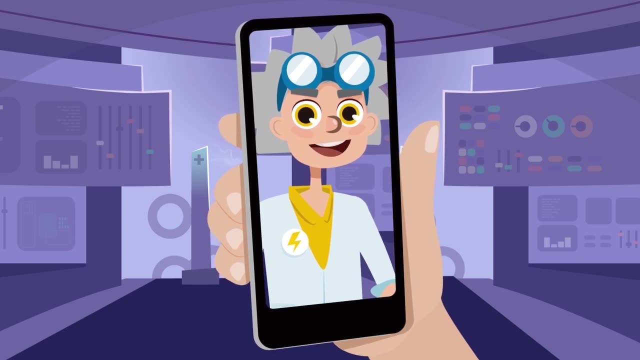 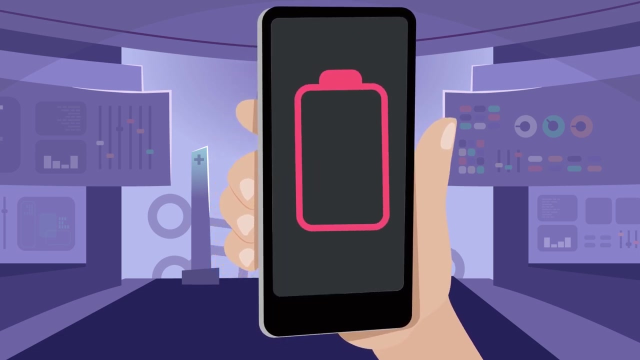 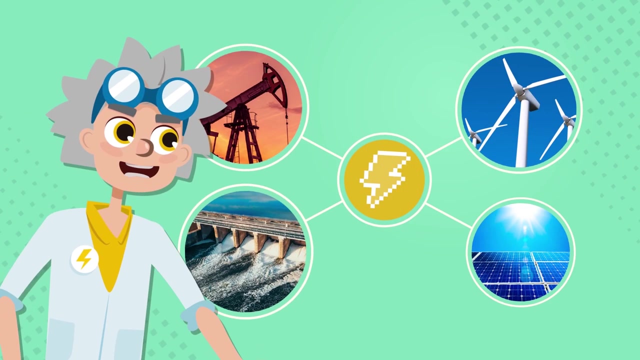 Now that we know what static electricity is, let's look at dynamic electricity. Static electricity only lasts a short time. Obviously, we can't use it to charge our cell phones or turn on a lamp. We need to obtain a different type of electricity using the natural resources around us. 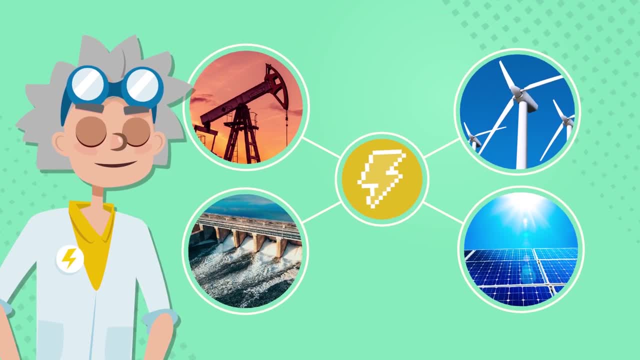 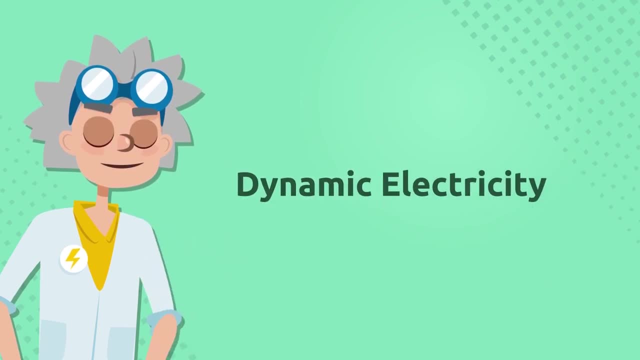 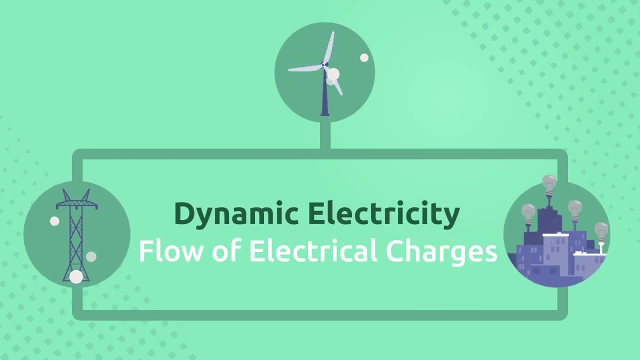 As I explained to you in our last video, the electricity we receive at home to run our house, to run our electronic devices, is called dynamic electricity. Dynamic electricity is the flow of electric charges. Just as water flows in a river, so do electrical charges in a cable. 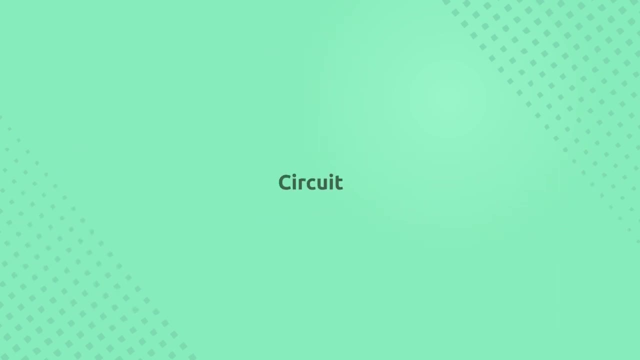 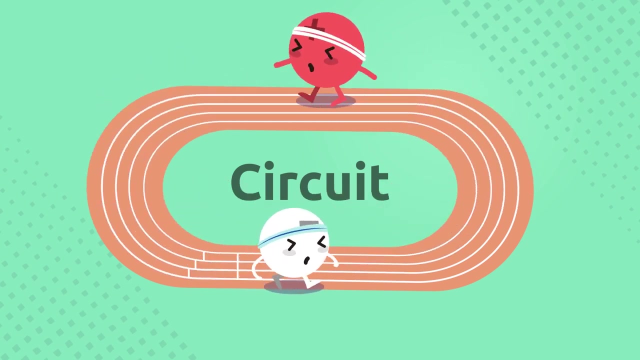 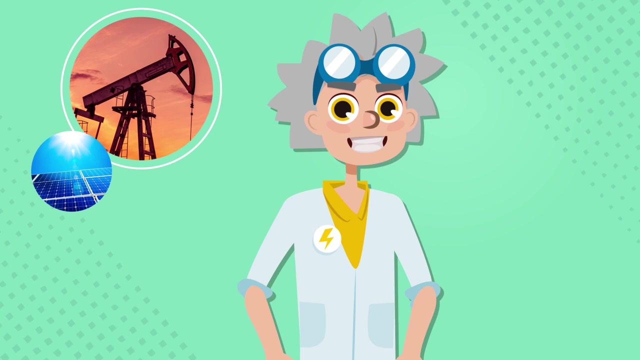 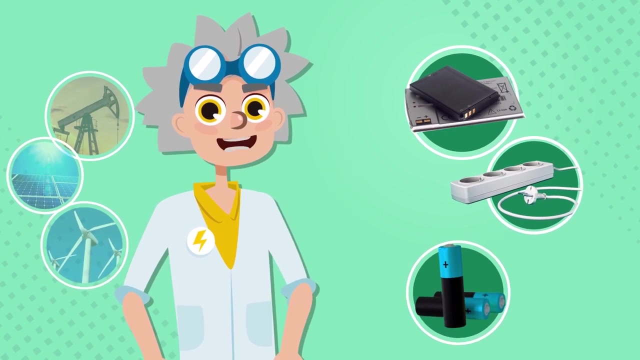 In order for electrical charges to flow continuously, we need a circuit. A circuit is a closed path in which electrical charges travel along. A circuit has two parts. The first is the source of electricity, which we discussed in the previous video, And the second corresponds to the materials that allow the flow of electric charges. 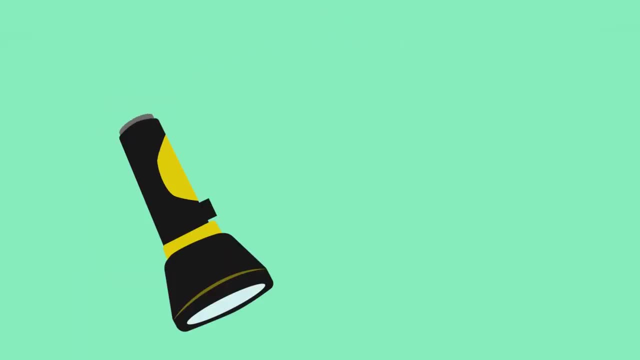 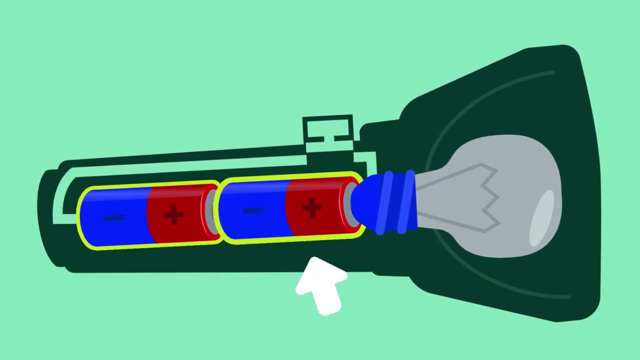 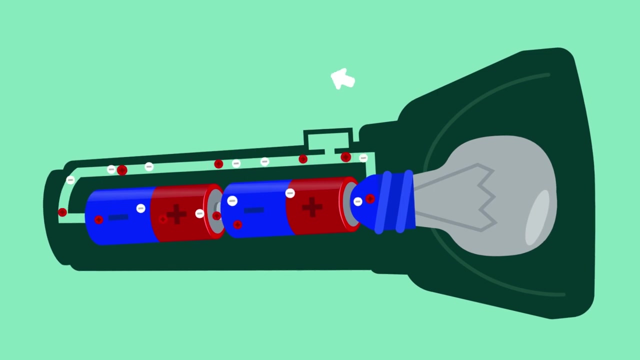 I'm going to show you Here. we see an electric circuit inside this flashlight. There are two batteries, which are the source of electricity, and the wires that carry the electric charge to the bulb. If I turn on the switch, the electric charges begin to flow through the wires and the bulb emits light. 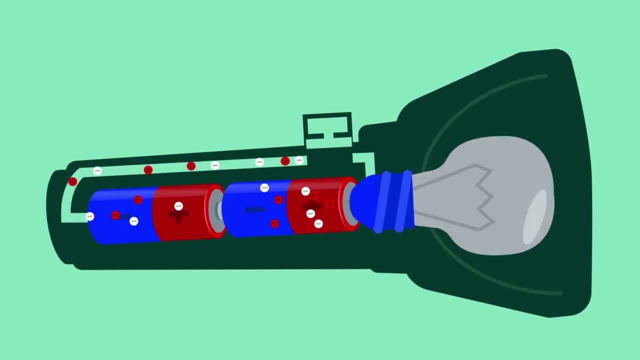 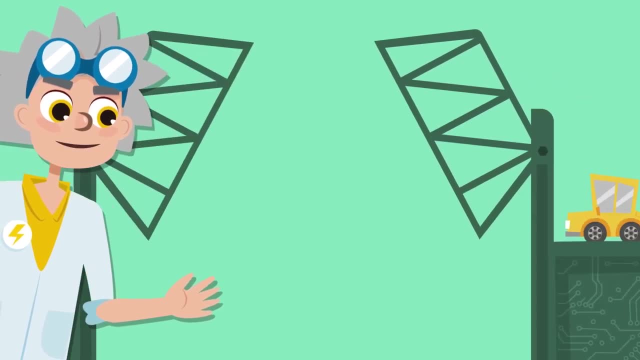 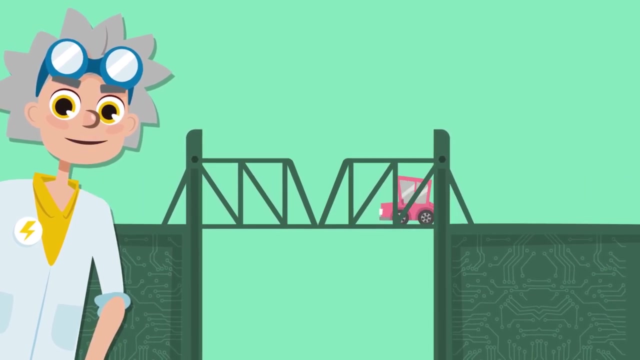 If I turn off the switch, the electrical charges stop flowing and the bulb stops emitting light. This works the same as a drawbridge. When its parts are lowered, cars can go back on the road. The same is true for the electrical charges in a circuit. 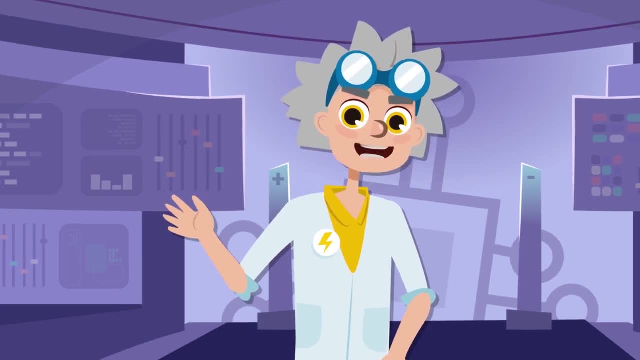 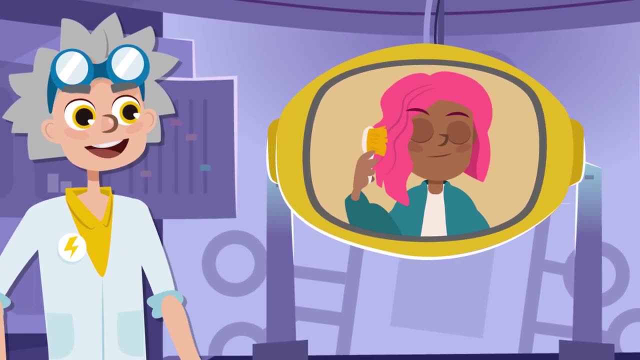 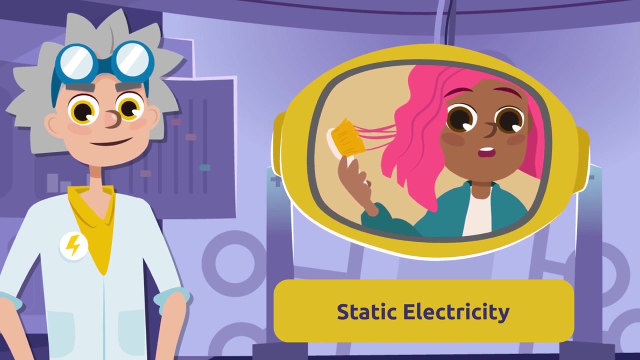 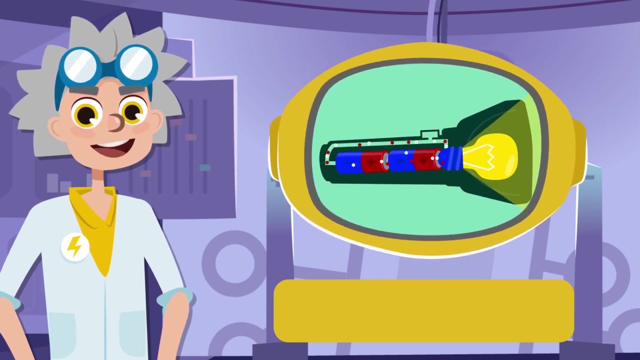 All right, guys. Now that we've learned all about the types of electricity and circuits, let's see what you remember. An imbalance of positive and negative charges between two objects is called Static electricity. Static electricity, That's it, And the flowing of electric charge is called 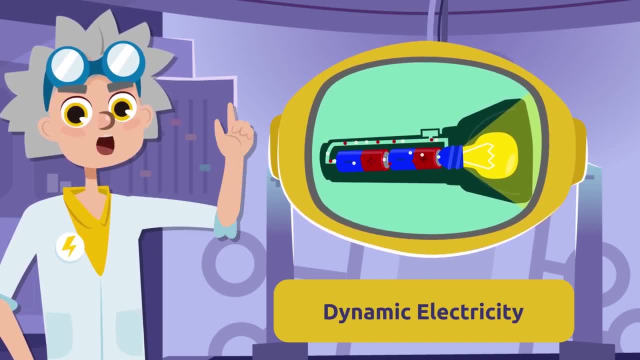 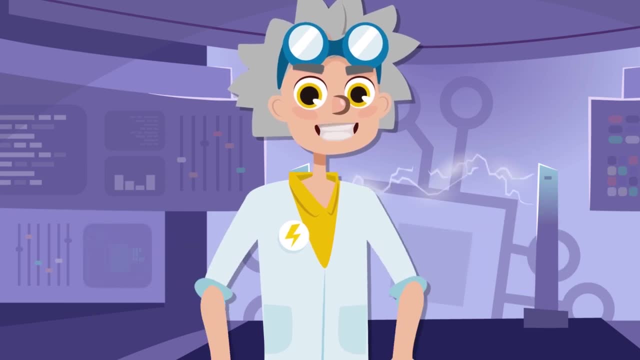 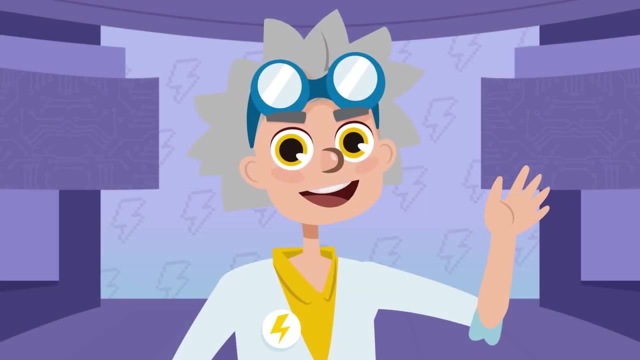 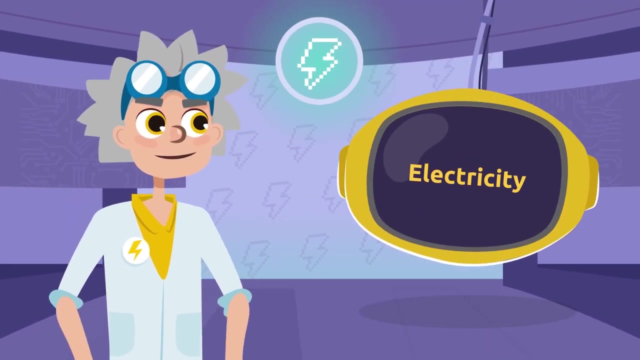 Dynamic electricity. Dynamic electricity. Very good, Great job. See you at the next show, Don't miss it. See you soon. Welcome back to Science Madness. In today's program we're going to learn more about electricity. We'll create an electrical circuit. 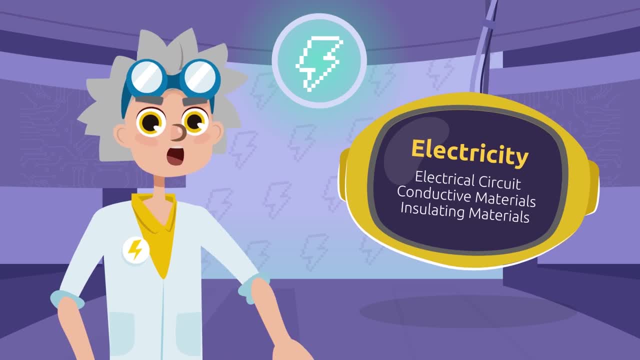 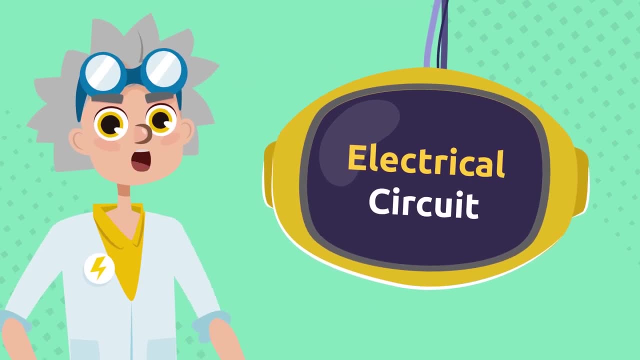 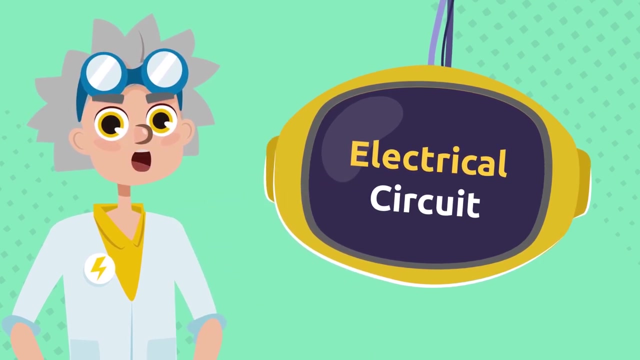 and we'll find out which materials are conductors and insulators Ready. We will start by building an electrical circuit which, as you know, is a closed path that electric charges flow through. I will need two wires, a light bulb, 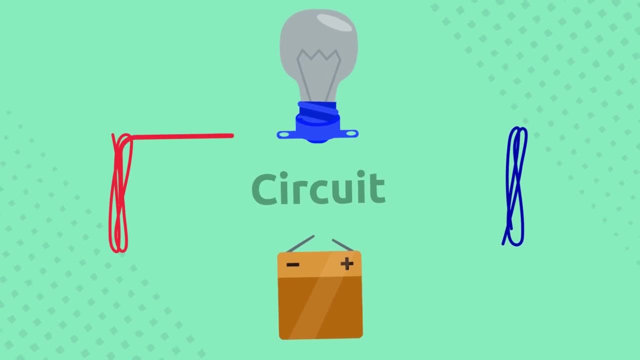 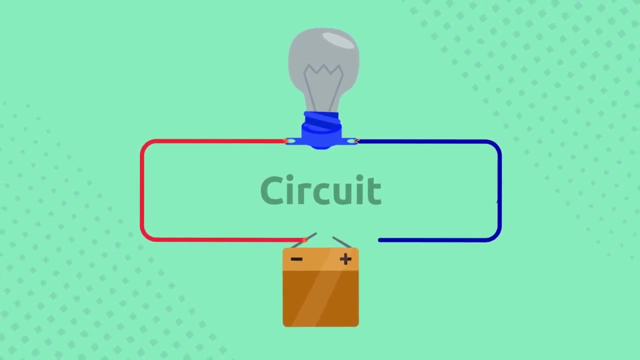 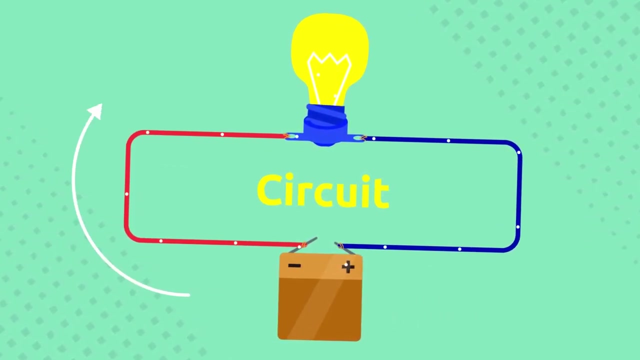 and a battery. We will attach one end of the wire to the light bulb and the other to one of the battery's end. I'll repeat the same steps with the other wire and Voila, We've just created an electrical circuit. The electric charges flow from the battery. 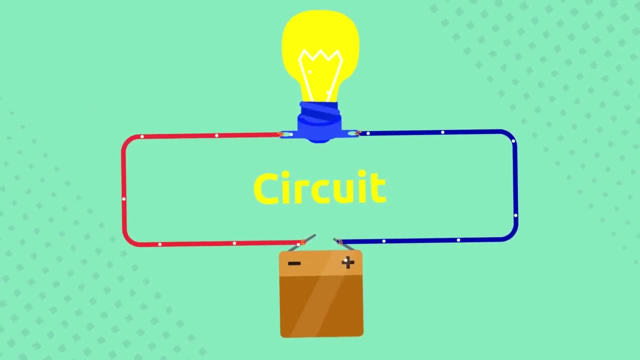 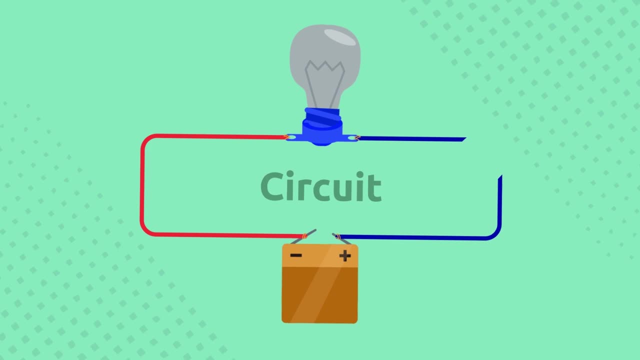 to the light bulb through the wires and, as a result, the light bulb lights up. Isn't it impressive. If I disconnect this circuit, the electric current stops flowing and the light bulb turns off. When I reattach the wire, the light bulb turns back on. 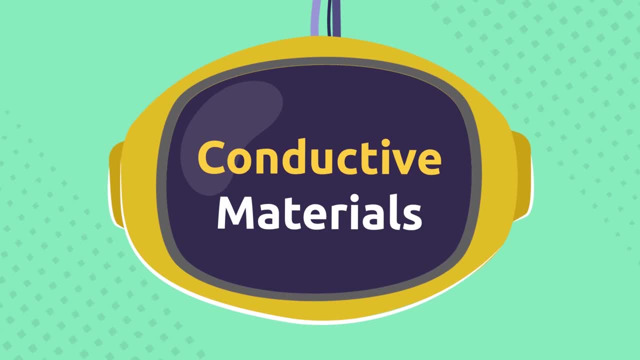 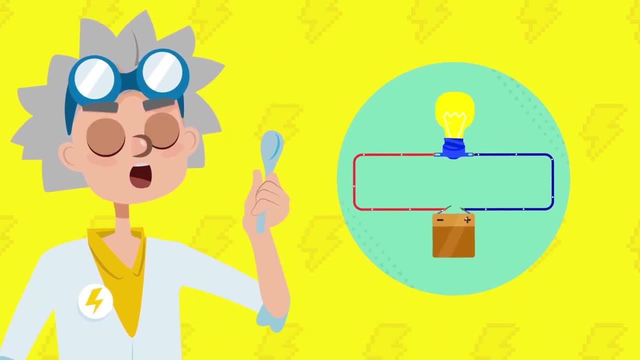 How cool is that? Let's see how it works. Let's see how it works. Let's make this more interesting. What would happen if I added this spoon to the circuit? Do you think the light bulb would still work? Would you like to make a bet? 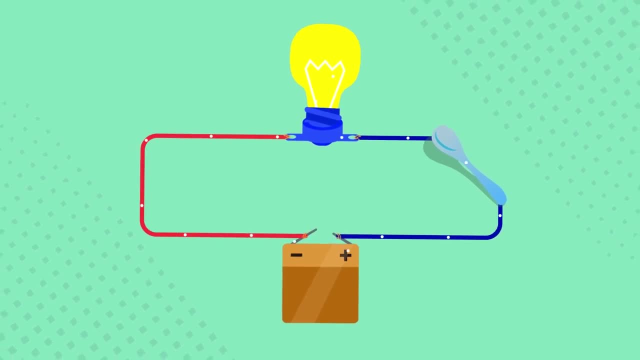 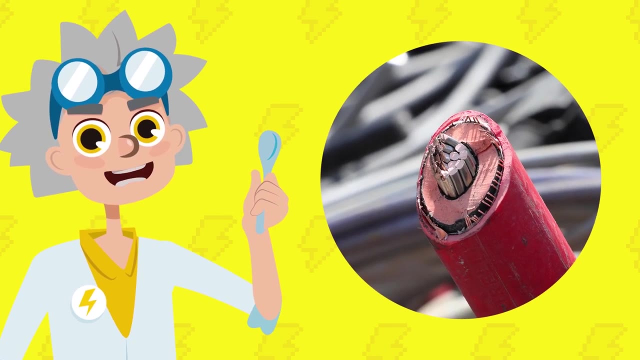 Ta-da, The light bulb came on. Amazing, isn't it? Just like the copper inside the wires. this spoon is made of metal, and metal is a great conductor of electricity. Silver, iron or aluminum are examples of conductive metals. 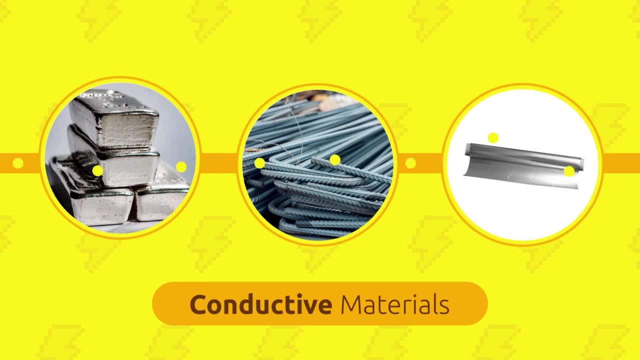 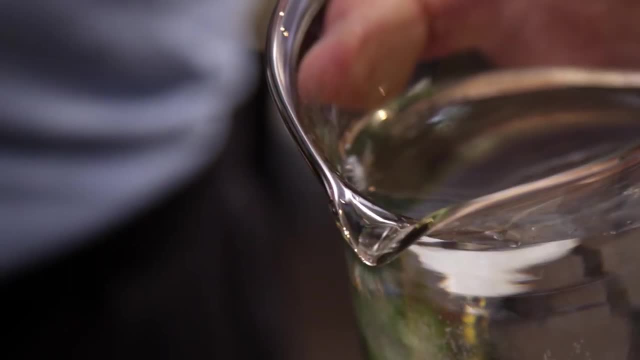 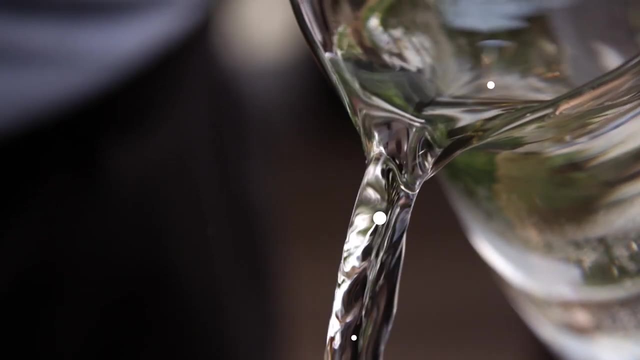 Conductive materials allow electrical charges to flow through them and therefore are the best materials to add to an electrical circuit. But conductive materials aren't only metals. Water, for example, is also a conductive material. Curious, isn't it. 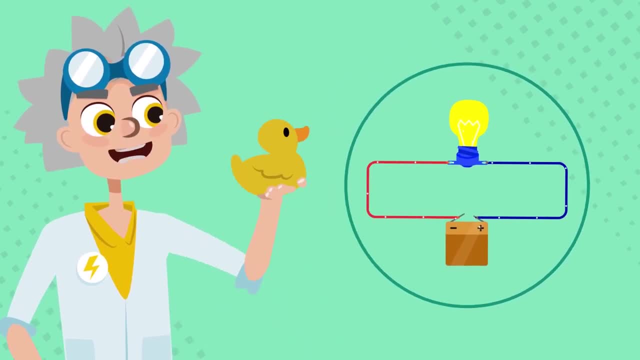 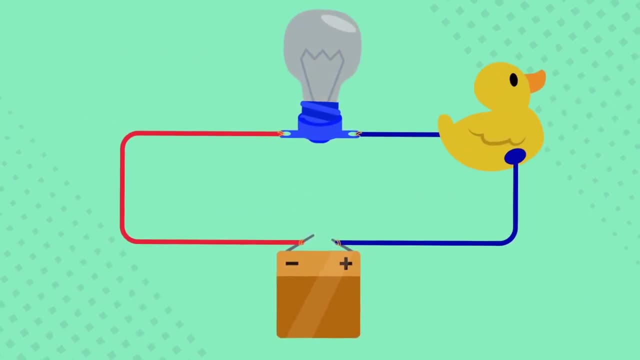 Let's try another type of material. Look at this rubber ducky. If we attach it to the circuit, what will happen? Will the light bulb turn on? Ooh, The light bulb didn't turn on. The little ducky is made of rubber. 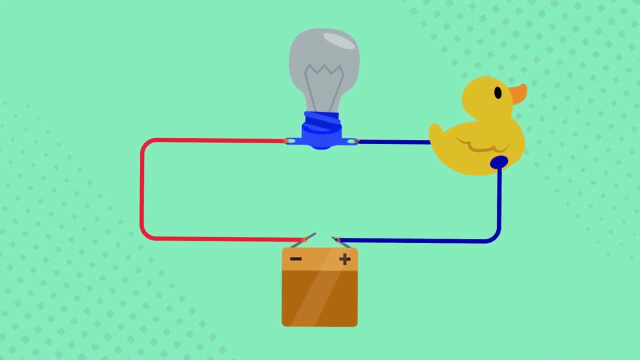 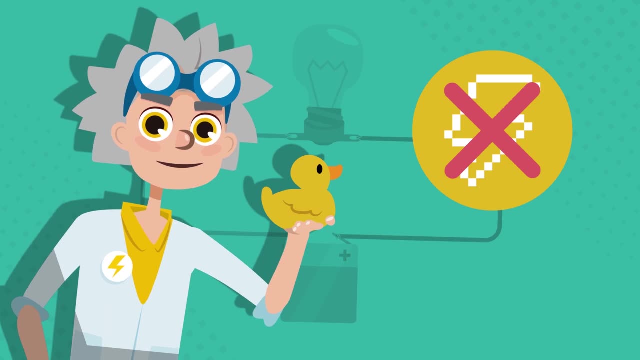 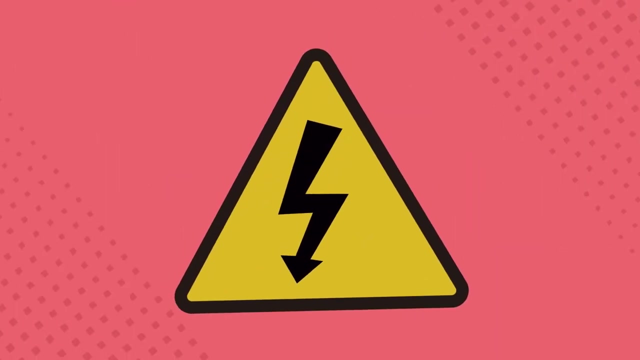 and rubber is an insulating material. Insulating materials do not allow electric charges to flow through them. That's why the light bulb didn't light up. Other materials such as paper, plastic or glass are also insulators. As you know, electricity can be very dangerous. 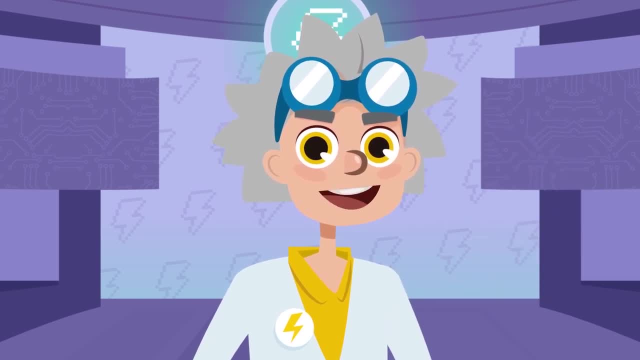 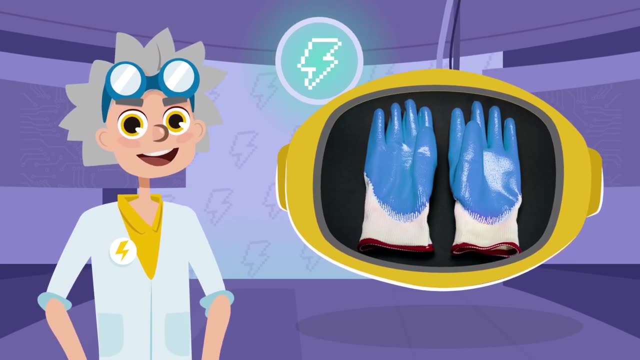 So insulating materials are used to protect us from it. For example, the outside of wires are made of plastic and electricians' gloves are made of rubber. Well, I think that's it, friends. I hope you had fun and, at the same time. 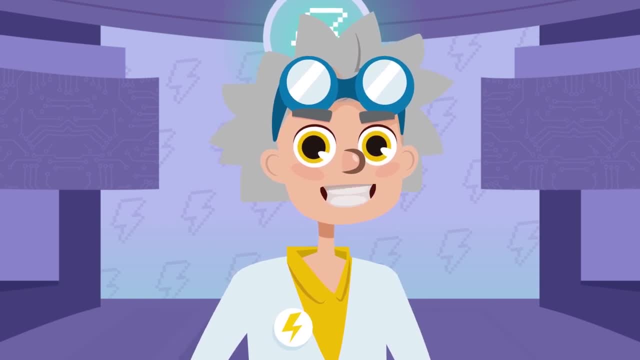 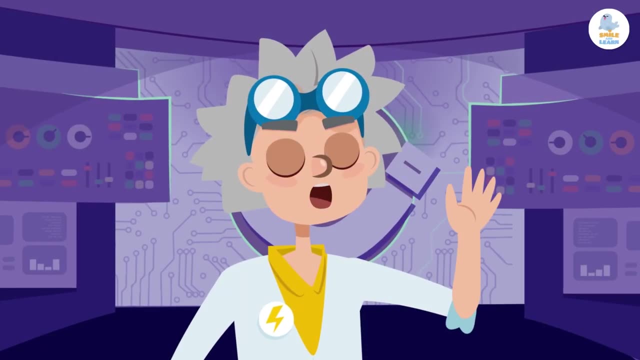 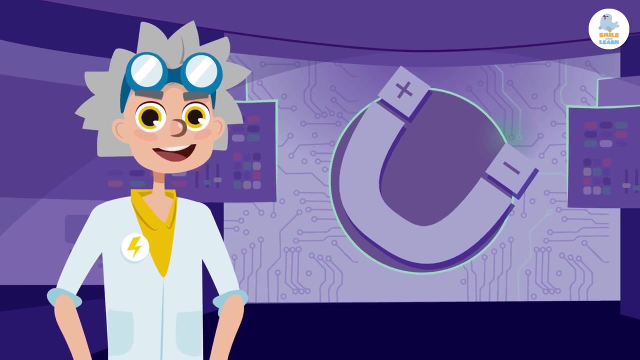 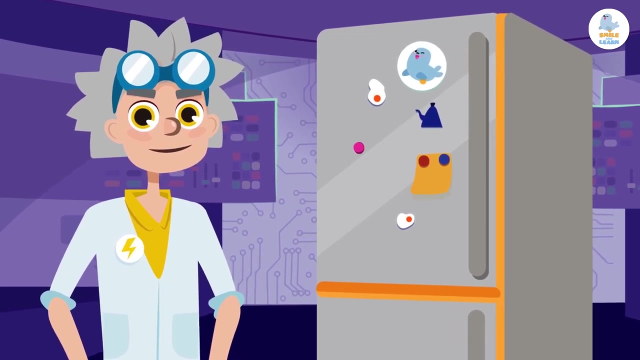 learned a lot of interesting things about electricity. See you soon. Welcome back to Science Madness. In today's program, we are going to learn about magnetism. Have you ever wondered why magnets stick to the fridge and don't fall off? This happens thanks to a property called magnetism. 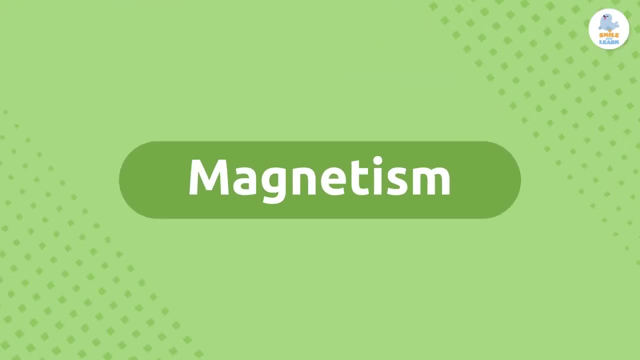 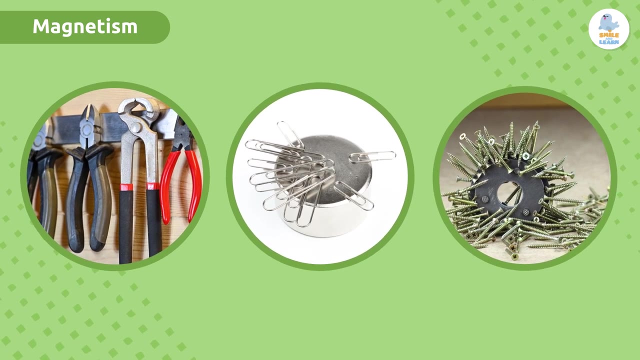 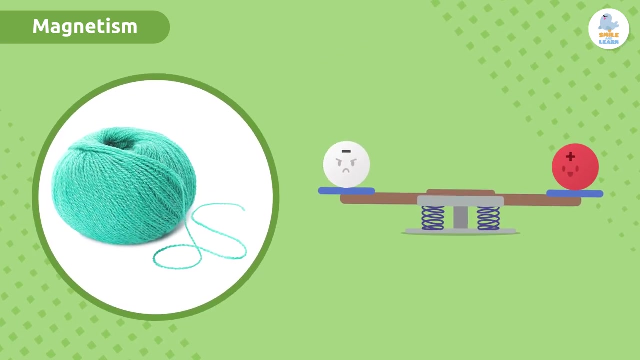 Let's see what it's all about. Magnetism is the property some objects have that attracts other metallic elements like iron. As you know, all matter has an electric charge. Normally this charge is electrically neutral, which means there is an equal number. 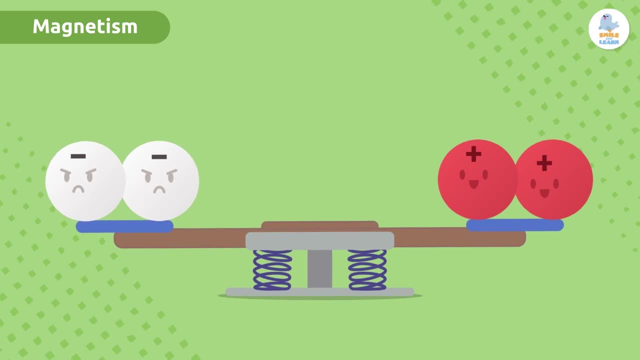 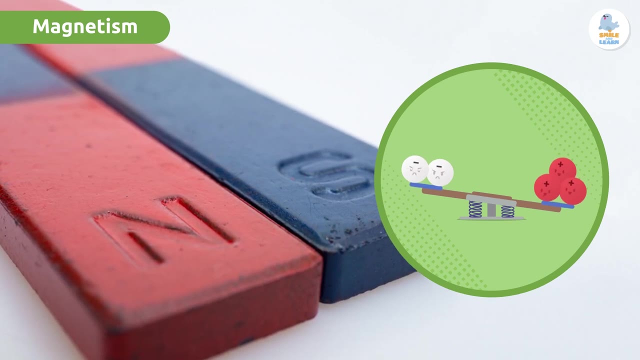 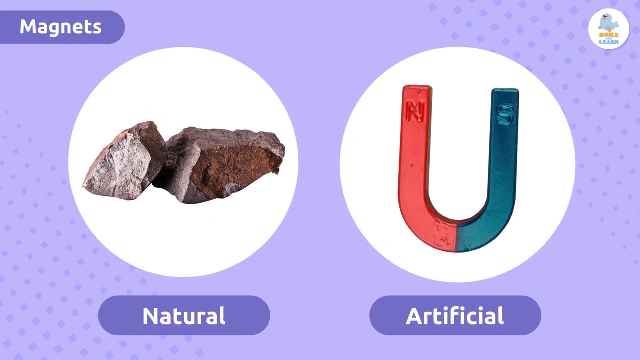 of negative and positive charges. However, in some materials this is not true, and this imbalance of charges causes attraction or repulsion. Magnets can be both natural and artificial. One of their main properties is the ability to attract objects made of iron and other metallic materials. 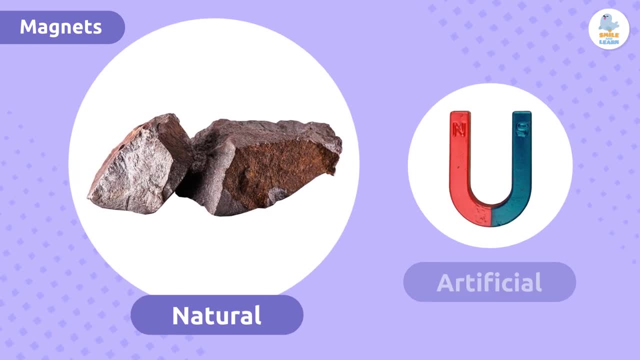 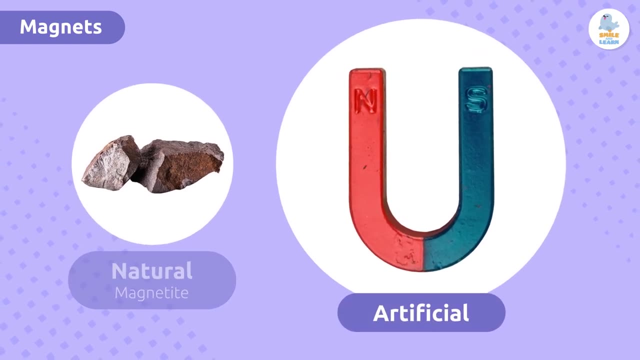 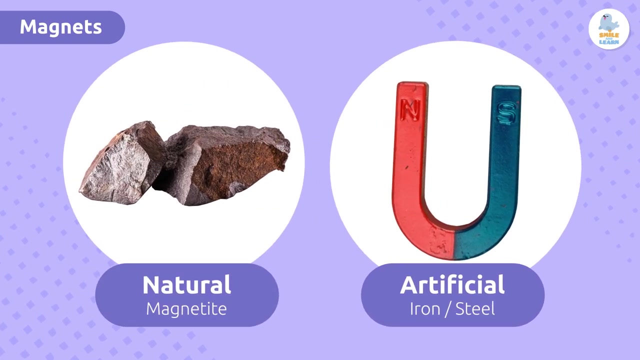 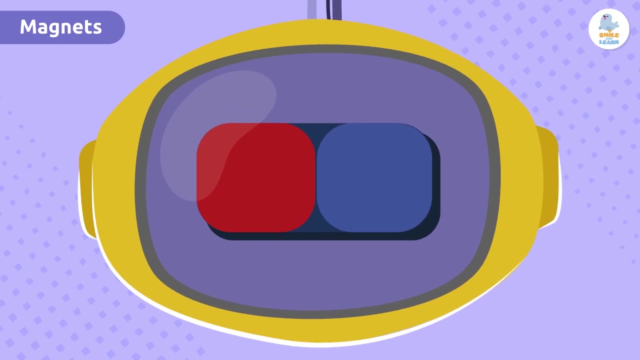 This is called magnetism. Natural magnets are found in nature. An example is magnetite. Artificial magnets are made by humans from different metals like iron or steel. So what are the characteristics of magnets? Come with me to discover them. Magnets have two poles. 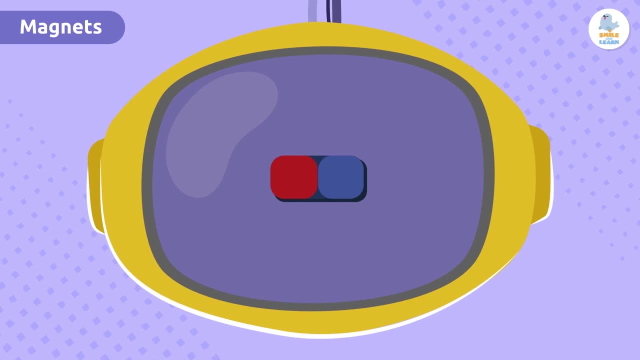 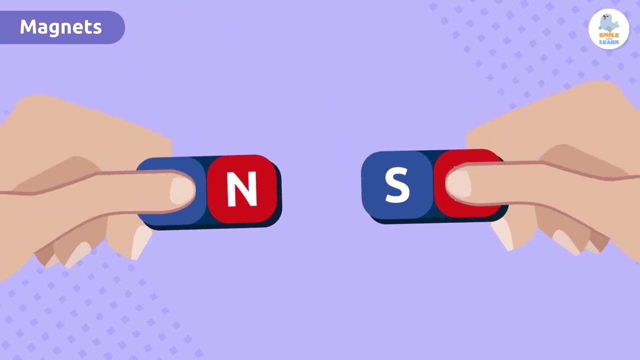 which we can find at their opposing ends. We call these ends the North Pole and the South Pole, and they generate a magnetic field. If we put two opposing poles together, they attract each other. This means that if we bring the North Pole of one magnet, 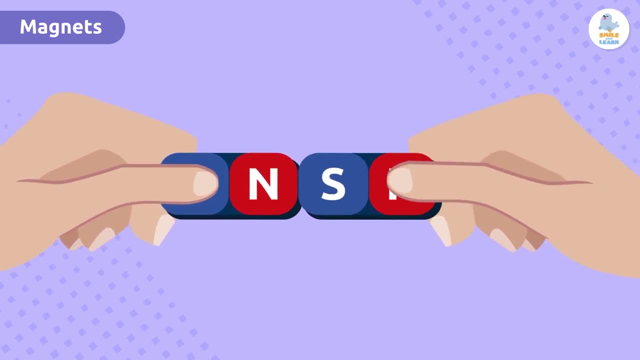 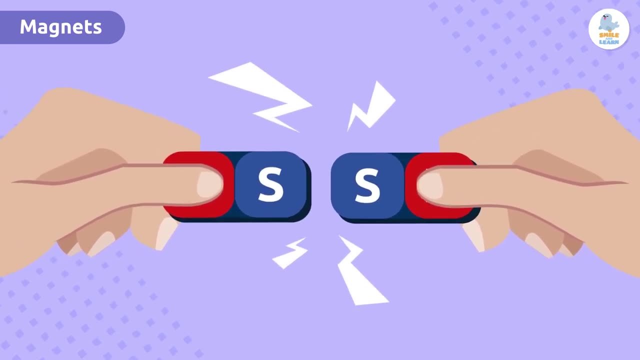 and the South Pole of another together, they attract each other. On the other hand, if we put two of the same poles together, they repel each other. Pretty interesting, right? But magnets aren't just used to hang the shopping list on the fridge. 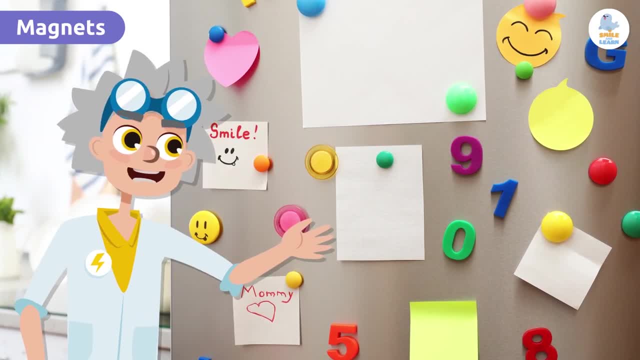 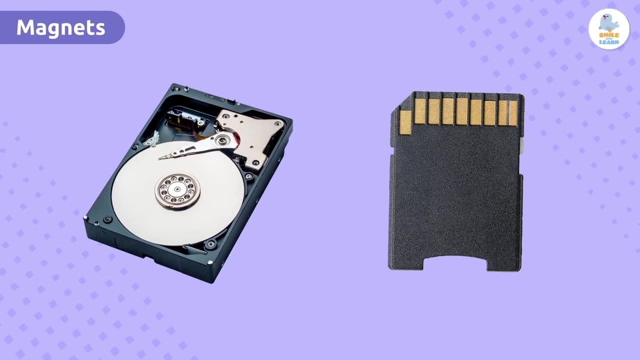 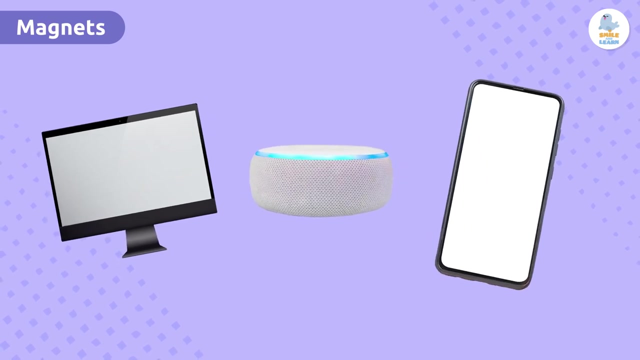 They can be used for many other things. Let's take a look at some examples. Digital storage devices such as hard disks and memory cards use magnetic properties to store data. Screens, speakers and other electronic devices also have magnets inside them. 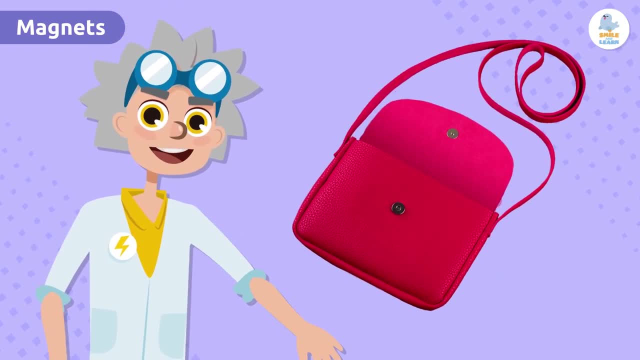 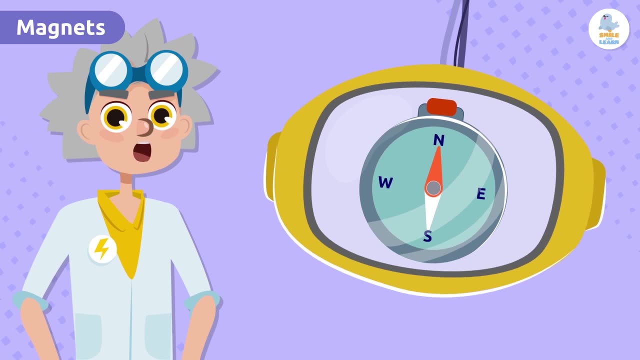 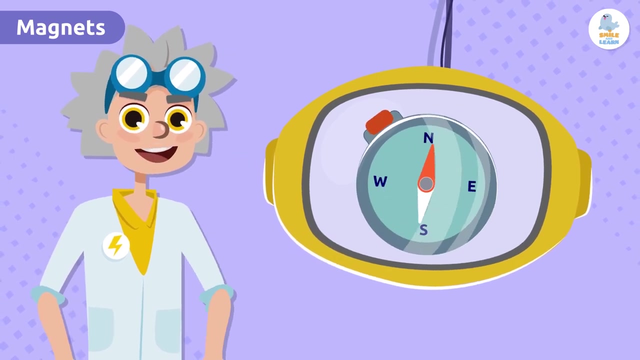 They're everywhere. I'm sure you've probably seen magnets on the clasps of bags and purses before right. Look closely. Did you know that compasses work thanks to magnets? Magnetism is very important in knowing our orientation and location. 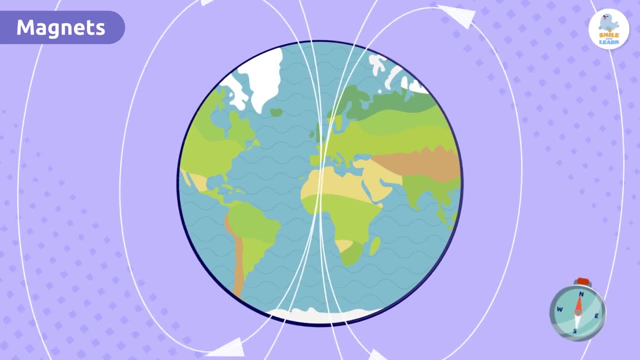 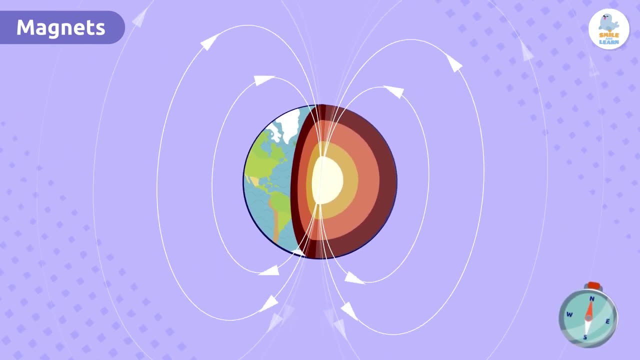 This is possible because our planet has a magnetic field that starts in the Earth's core, which is made up of metals such as iron and nickel, and extends through hundreds of miles of outer space. This magnetic field has a North and a South Pole. 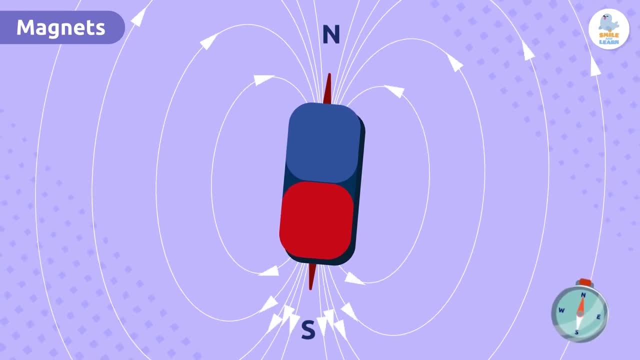 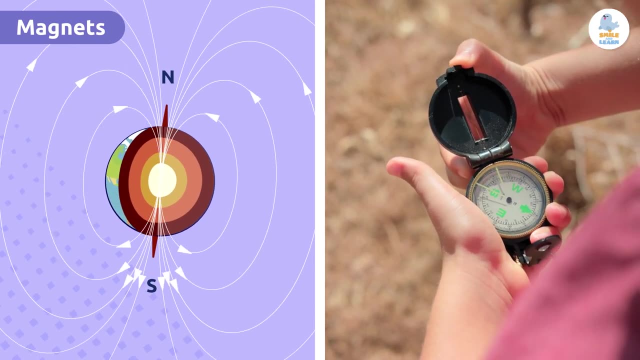 just like magnets. Because of this, we can say that the Earth acts like a giant magnet. It moves the compass needle to the North and allows us to know where we are, so we can move around without getting lost. Interesting, isn't it? 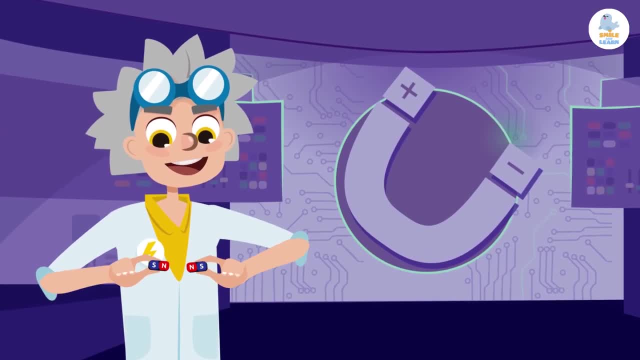 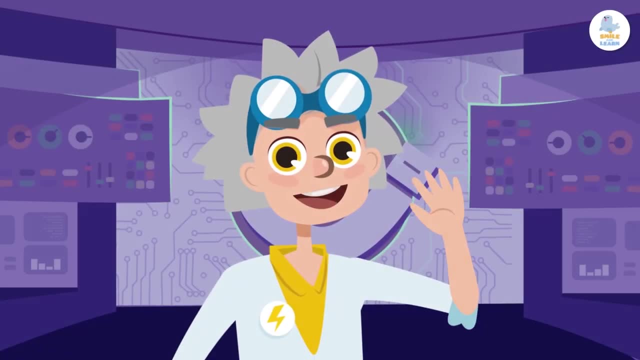 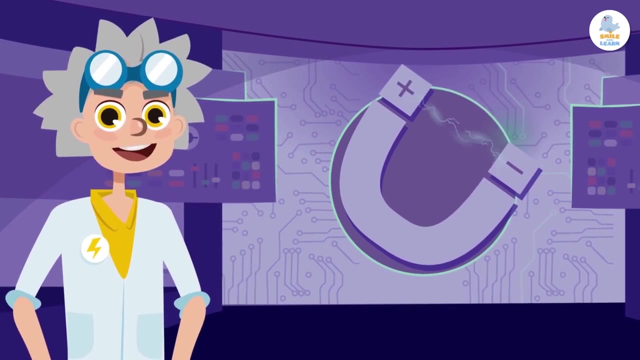 Good job, my friends. I hope you like magnets as much as I do. See you in the next video. Bye-bye, Welcome back to Science Madness. In today's video, we're going to learn about a very special type of magnetism. 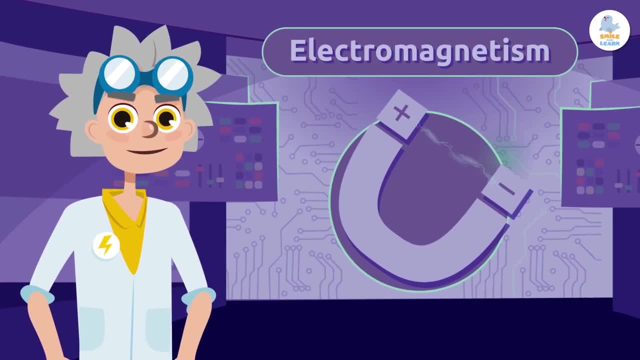 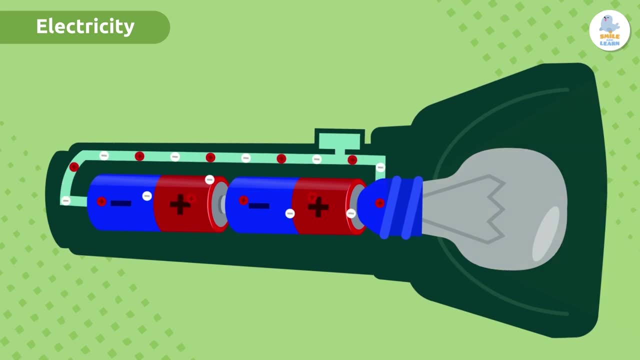 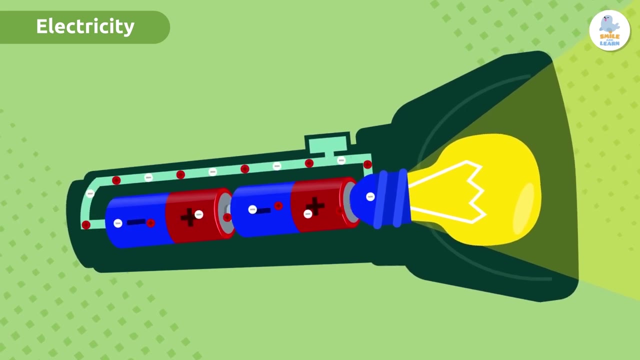 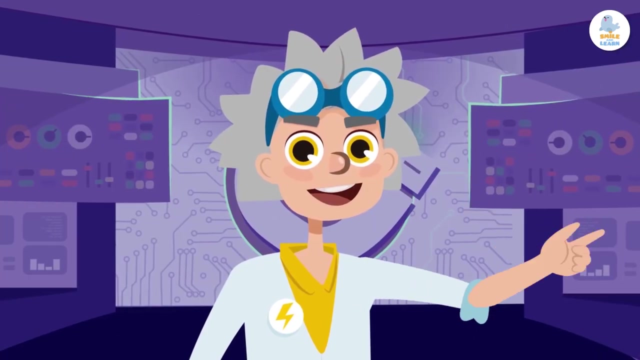 electromagnetism. First, let's review what electricity is. Electricity is a physical phenomenon that occurs when there is movement of electrical charges in objects. This is called an electrical current. These electrical charges can be positive or negative. Now that we have reviewed what electricity is, 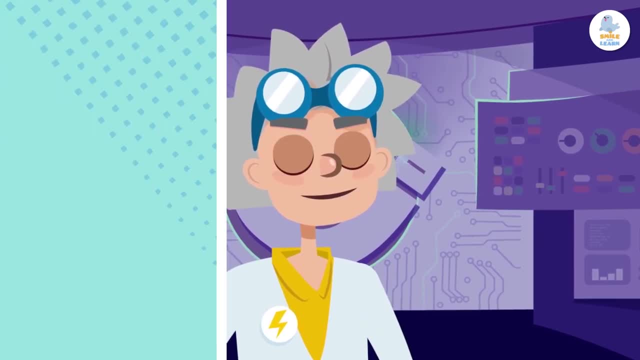 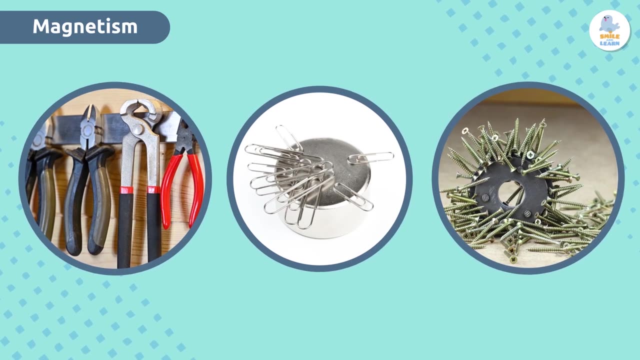 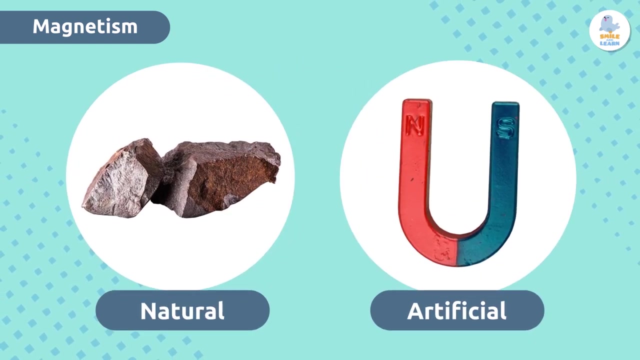 do you remember what magnetism is? Magnetism is a very interesting property that some objects have. It causes them to attract metallic elements like iron. These objects are called magnets. They can be natural or artificial and have two magnetic poles: the North Pole and the South Pole. 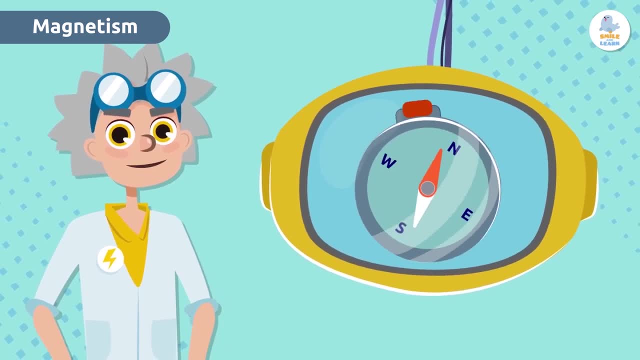 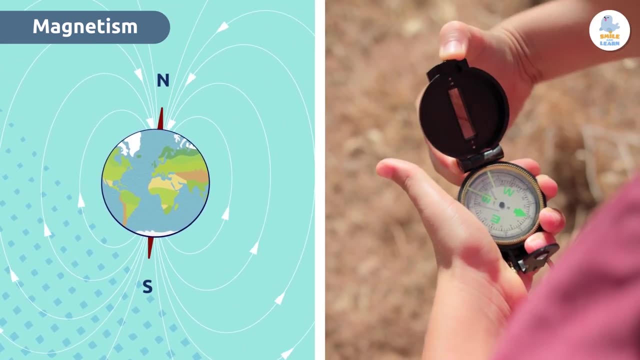 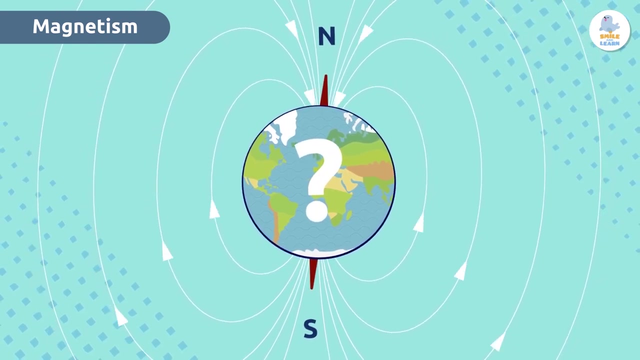 Have you ever used a compass to orient yourself? A compass uses a magnetized needle that always points to the Earth's magnetic North Pole, which allows us to locate ourselves on a map. And do you remember what a magnetic field is Exactly? It is the space surrounding a magnet. 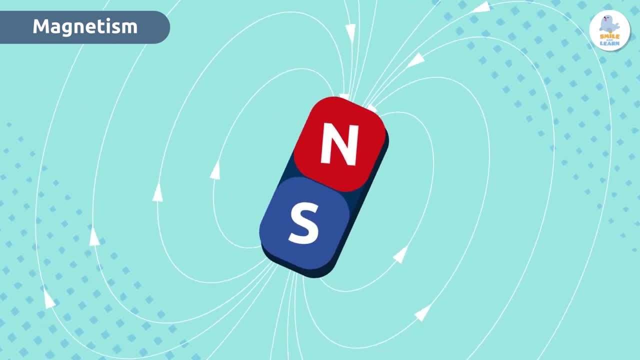 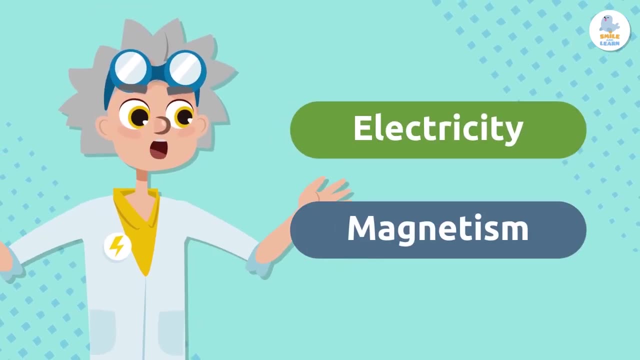 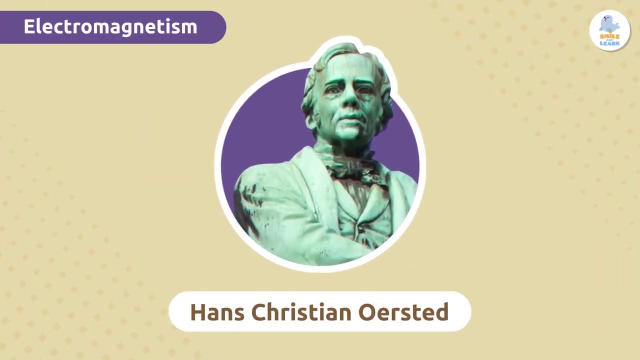 where its magnetic force acts. In other words, it is the space where a magnet can attract other metals. Now we are ready to learn what electromagnetism is. Here we go. Let's start with a bit of history In the 19th century.